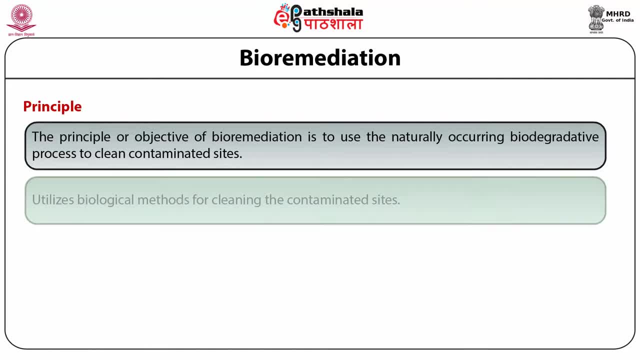 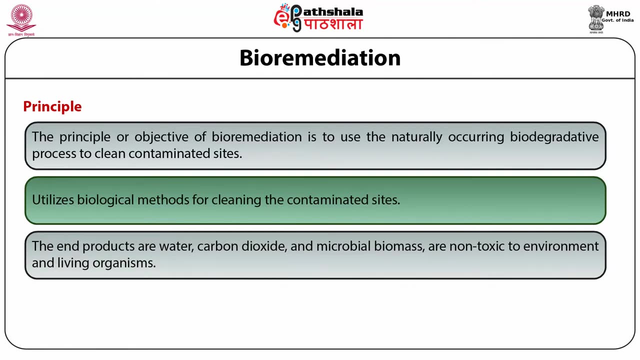 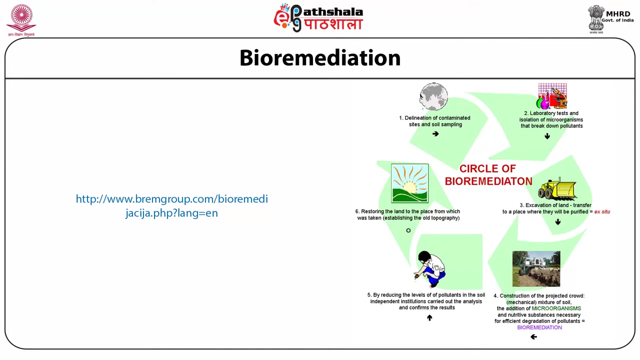 Hence the bioremediation process utilizes biological methods for cleaning the contaminated sites, including soil, water, air. The end products of bioremediation, such as water, carbon dioxide and microbial biomass, are non-toxic to environment and living organisms. Here in this picture shows the circle of bioremediation, which starts from the delineation of contaminated sites and soil sampling. 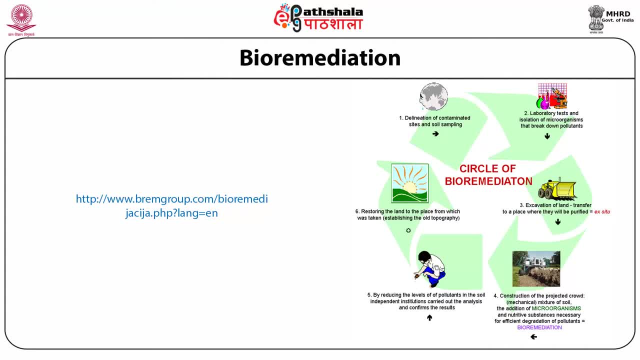 Then the laboratory test and the isolation of microorganism that break down the pollutants. carried out bioremediation In the laboratory section, then, after that, excavation of the land, then the transfer to a place where they will be purified. This method is comes under the ex-situ remediation method. 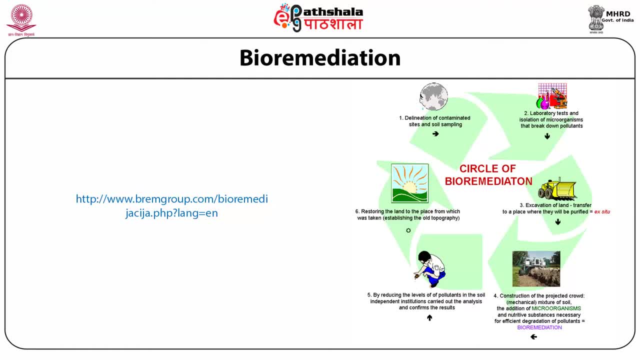 Then the next step, including the construction of the projected crowd mechanical mixture of the soil. The addition of microorganism and nutritive substances After the bioremediation compounding and medium organization is necessary for efficient degradation of pollutants. that is known as bioremediation. 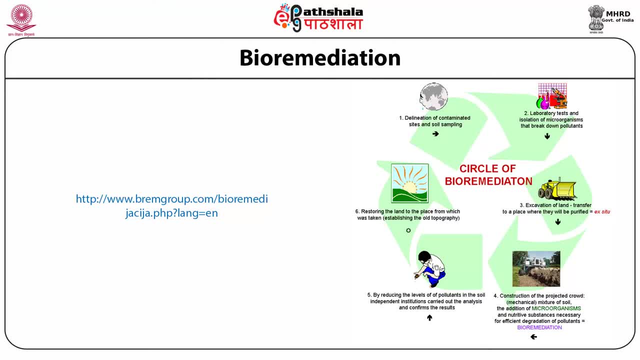 After the bioremediation, by reducing the level of pollutants in the soil. independent institutions carried out the analysis and confirmed the result, Then restoring the land to the place from which it was taken, Establishing the old tropical Bronze. So the whole circle is start, from the identification to the reestablishment of the natural condition done by the bioremediation processes. 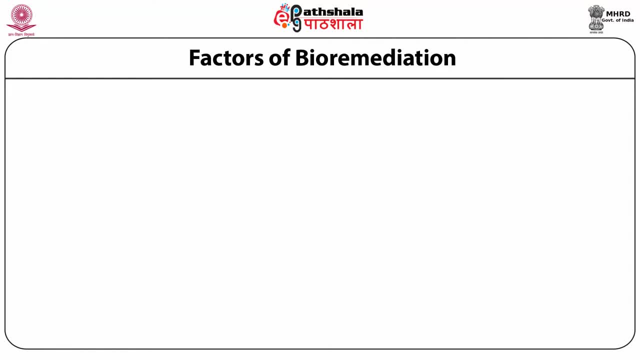 Now discuss about the factors of bioremediation. The control and optimization of bioremediation processes is a complex system of many factors. These factors include the existence of a microbial population capable of degrading the pollutants. the availability of contaminants to the microbial population. 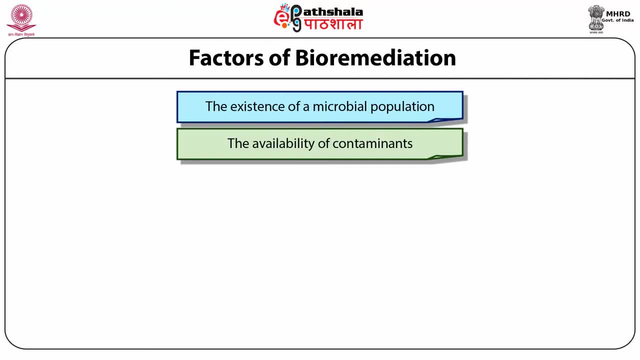 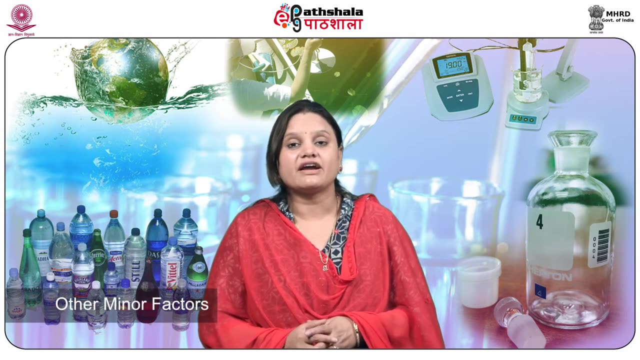 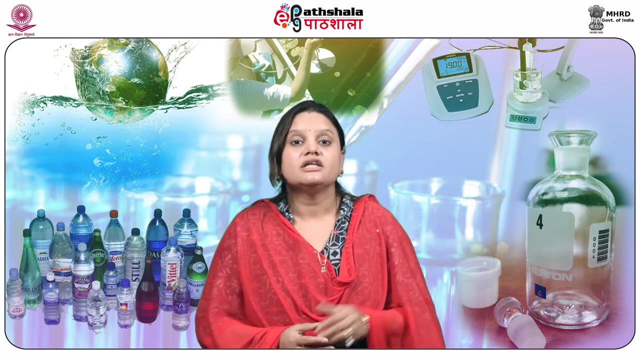 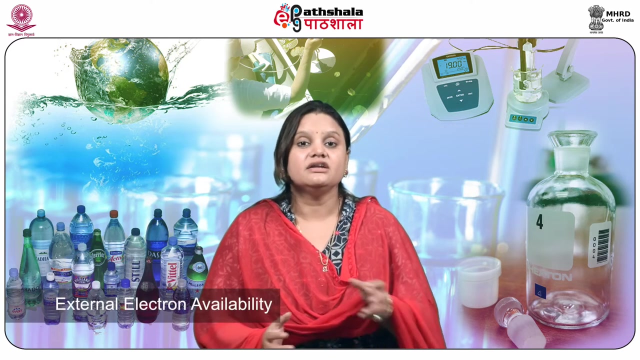 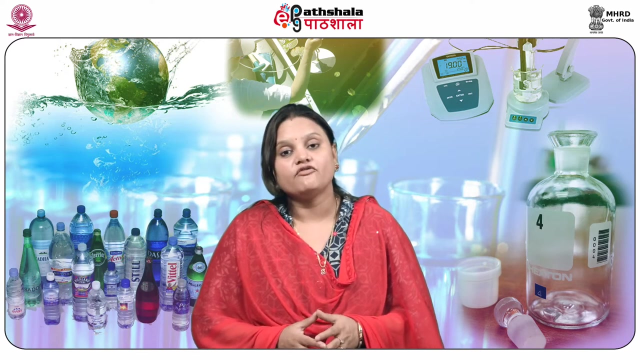 then the environmental factors, like types of soil, temperature, pH, the presence of oxygen or other electron acceptors and nutrients, The other minor factors of bioremediation, including the contaminants, type and its concentration, water content and geological characteristics, nutrients availability, external electron availability, soil type, temperature, bioavailability of pollutants, co-metabolism, gene expression and the type of microorganism. 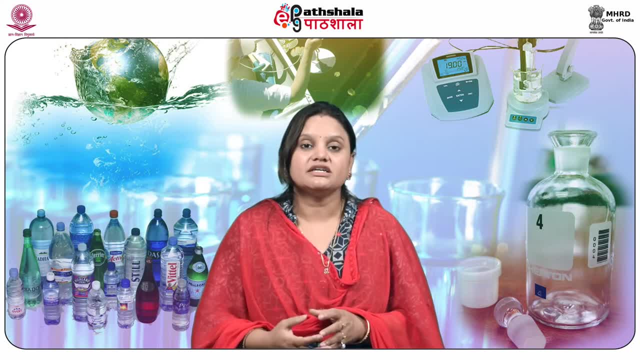 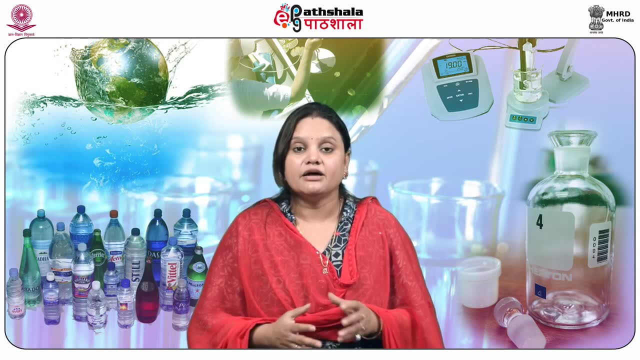 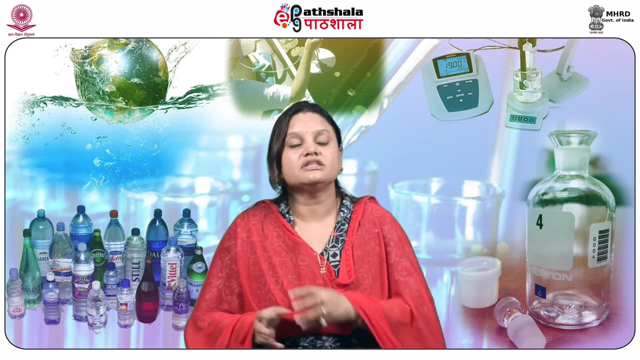 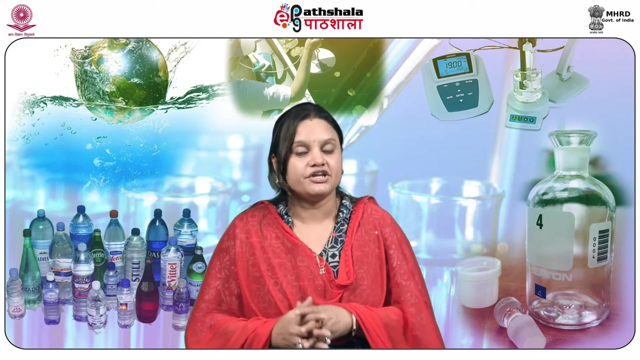 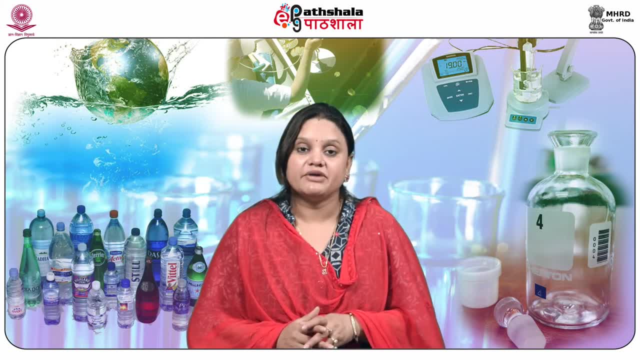 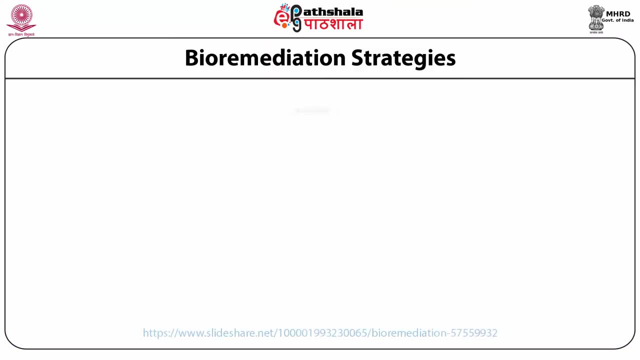 And the third. one type of bioremediation is known as phytoremediation, which is done by growing the plants. Now, in this figure, we have discussed about the bioremediation strategies. Bioremediation is done by the two processes. 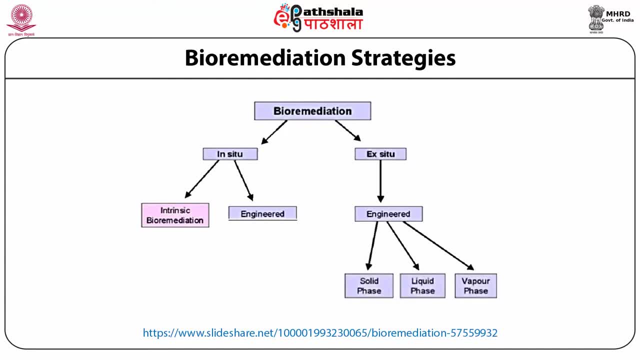 The number one is in-situ bioremediation. Number two is the ex-situ bioremediation. The in-situ bioremediation is done by intrinsic bioremediation. The in-situ bioremediation is done by intrinsic bioremediation and engineering practice. 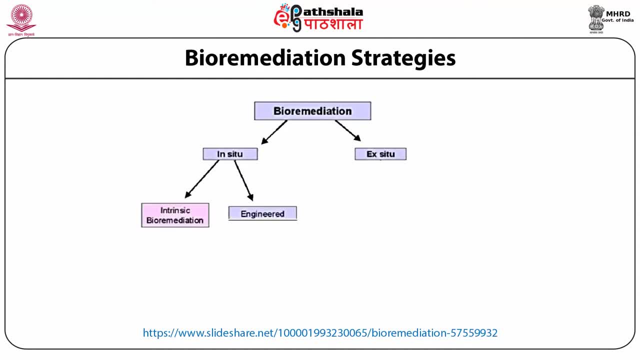 And the ex-situ bioremediation is only done by engineered practices, which include solid phase, liquid phase and the vapor phase. Now we are discussing here the techniques of bioremediation. The bioremediation carries on site or in-situ bioremediation. 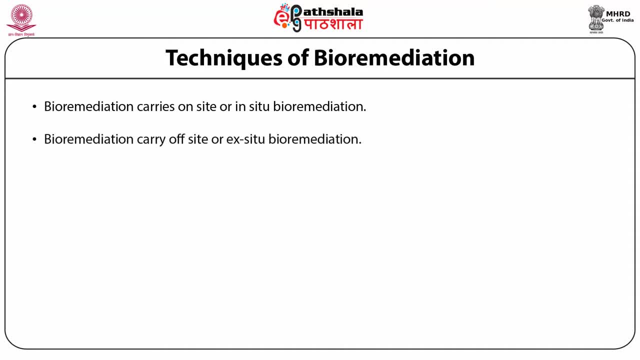 The next one technique is the bioremediation carries on site. Number one: we have discussed that bioremediation carries on site The Bombs. only unity is primary treated and the end-situ bioremediation is only done on site. 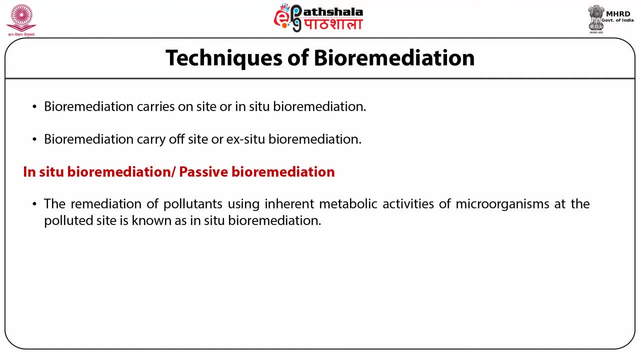 The êch Phoene de livres. hi glut formingy can only be Britney in off-site or ex-situ bioremediation. Number one: we are discussing here about the in-situ bioremediation, and it is also known as passive bioremediation. The remediation of pollutants using inherent metabolic activities of microorganism at the polluted site is known as in-situ bioremediation. When the microorganism are soluble as store in a side of the Earth, the Biotase removed. Then by doing these two, it can be girl. 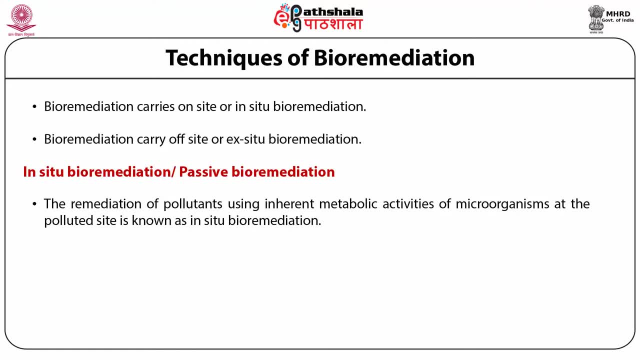 added or exposed to the pollutants. they degrade the pollutants as a result of their metabolic activity. the growth of microorganism and their ability to bring bioremediation are dependent on the supply of essential nutrients in situ. bioremediation has been successfully applied for the cleaning of oil spillage. 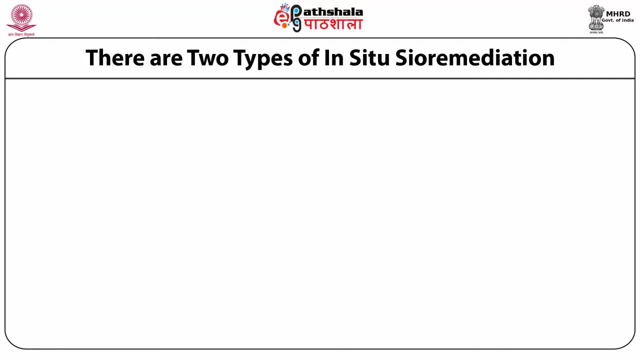 there are two types of in situ bioremediation technique. it includes intrinsic in situ bioremediation and accelerated or engineered in situ bioremediation. first of all, we have discussed here about the intrinsic in situ bioremediation: the remediation of pollutants using inherent metabolic 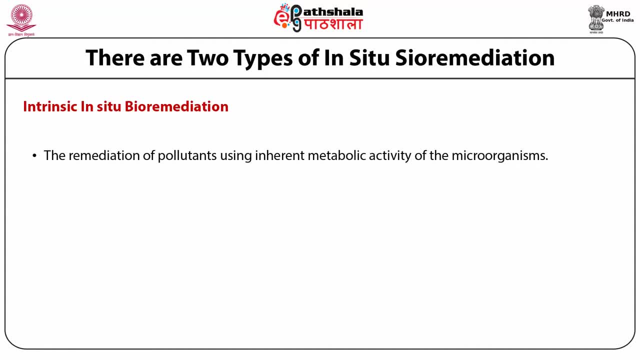 activity of the microorganism using the unique metabolic activity of the microorganism using the no Caedric, Actually indigenous- microbes is known as intrinsic bioremediation. The microorganisms may be tested at the laboratory for their natural capability of the biodegradation. 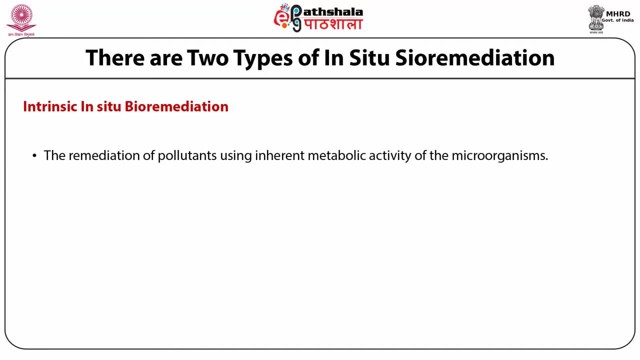 and appropriately utilized. However, the microorganisms or the site of which the pollutants are to be removed are not manipulated. The second procedure is accelerated or engineered in-situ bioremediation. It is the in-situ bioremediation in which the nutrients or substrates are added to the site. 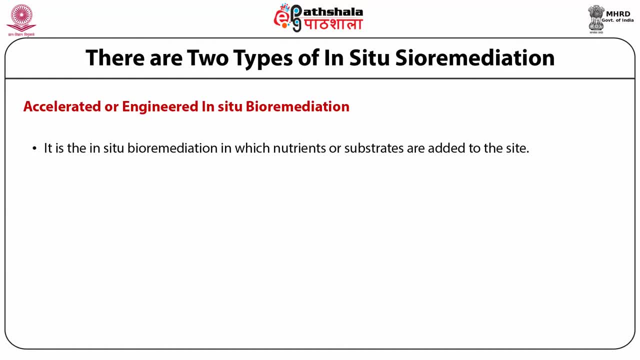 for example, oxygen, lactate nitrate, etc. or the environment is modified to stimulate the growth of microorganisms to increase the rate of degradation. The microorganisms may be indigenous. However, the microorganisms that highly efficient at degrading the pollutants may be introduced at the site. 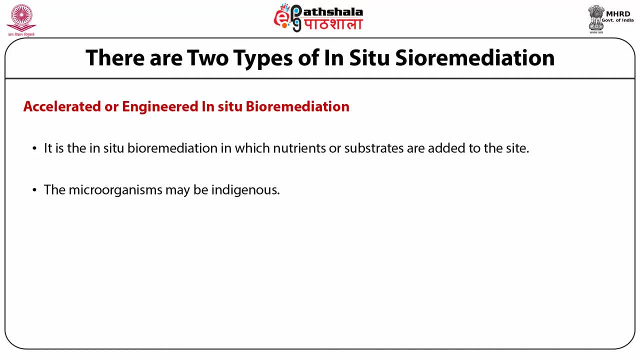 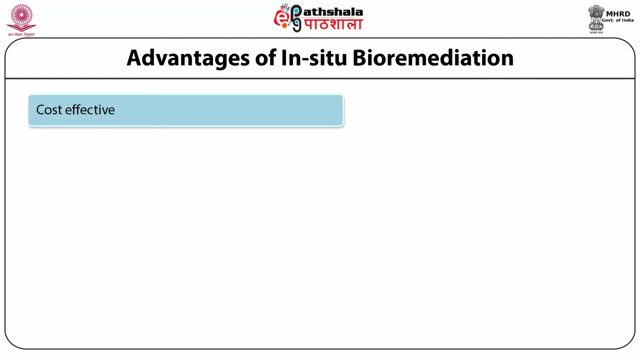 The accelerated in-situ bioremediation is used where it is desired to increase the rate of degradation. The microorganisms may be genetically modified. Thank you. The advantages of using in-situ bioremediation, including the cost-effective method, that this method is considered a very cheap and cost-effective method. 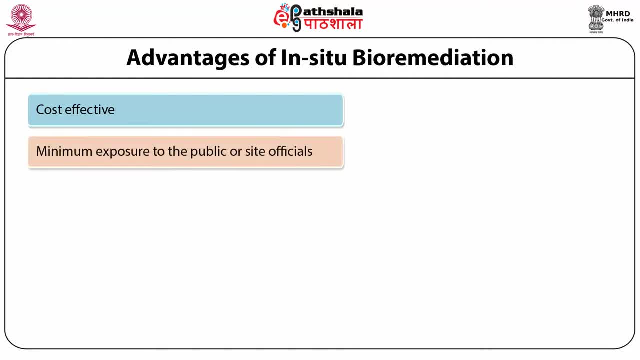 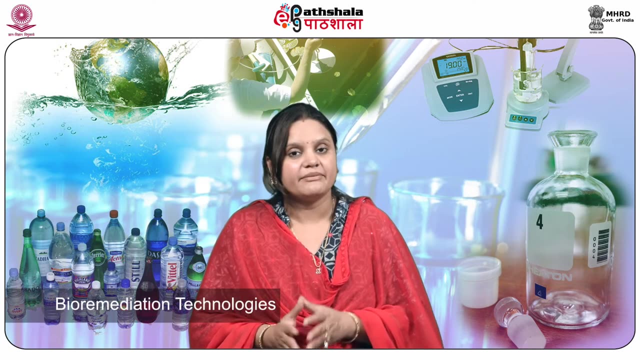 and the second one is the minimum exposure to the public or the site officials, and the site of remediation remains minimally disrupt. Now here we are discussing about the bioremediation, The bioremediation technologies. It is divided in in-situ and ex-situ techniques. 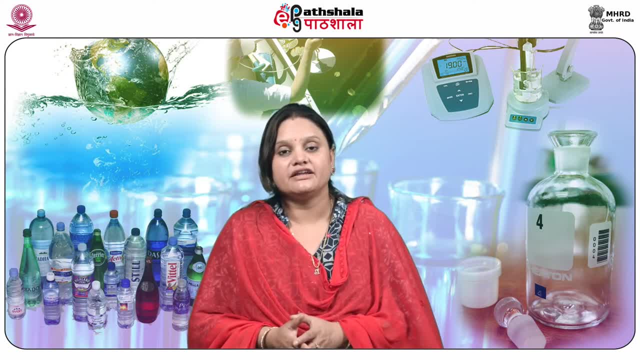 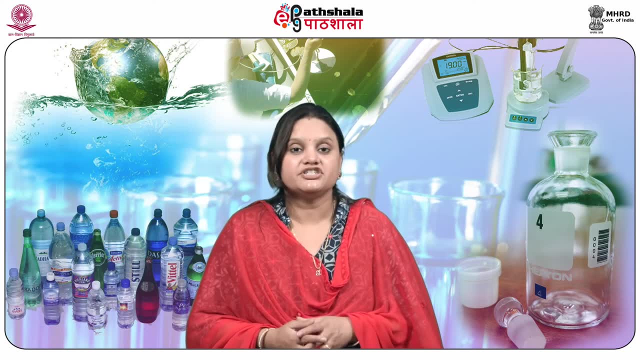 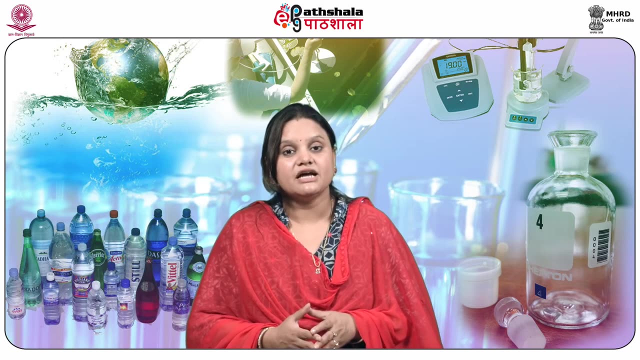 Under the in-situ bioremediation technique. it included bioventing, bio-stimulation, bio-augmentation, air sparging and the natural attenuation Number one. we are discussing about the bioventing. The bioventing is an in-situ bioremediation technique. 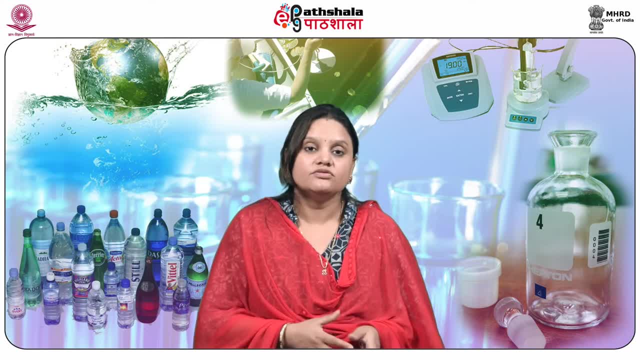 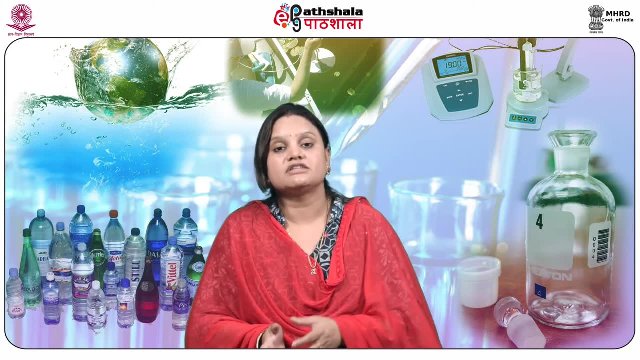 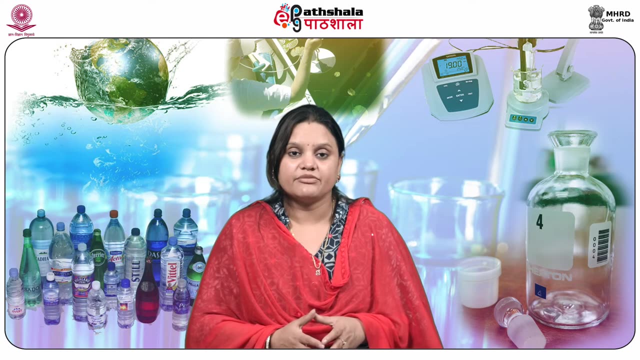 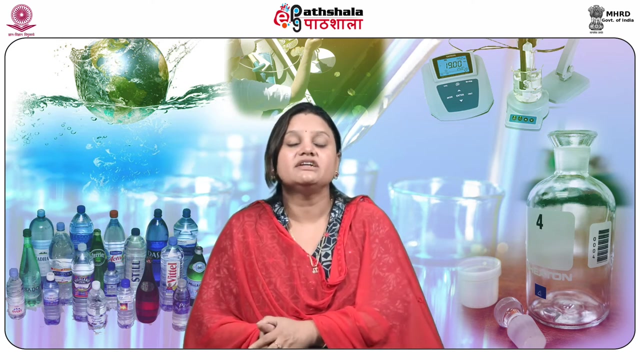 It is an in-situ bioremediation technique that uses indigenous microorganisms to degrade the pollutants in soil or the subsurface area In bioventing wells are made at the point of contamination or pollution, above the water level through which air or the nutrients are injected. 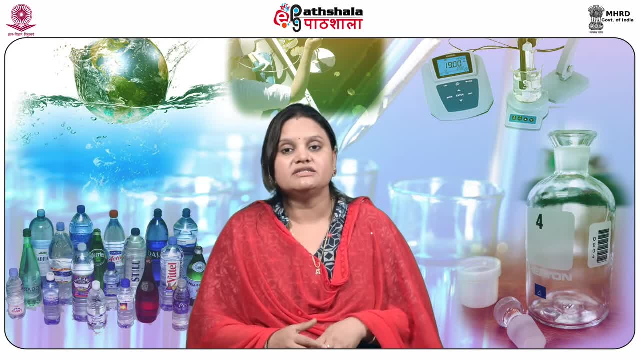 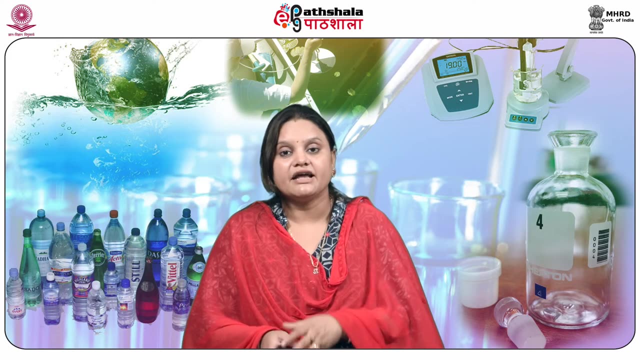 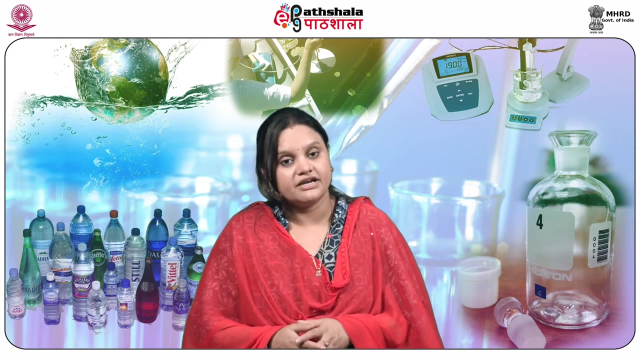 The microorganisms degrade the pollutants and the degraded pollutants are extracted from the extraction well and safely vented. The injection of air oxygenate contaminated soil and the contaminating material or the pollutants are biodegraded. The bioventing has been proved to be very effective. 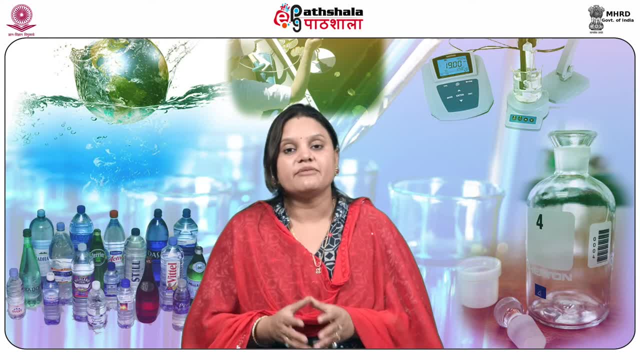 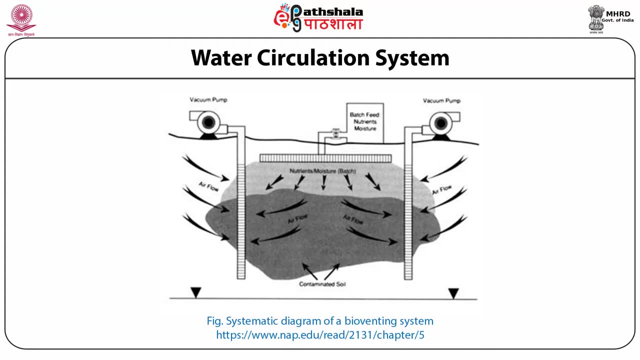 and remediating petroleum contaminated soil. Here in this figure, we are discussing about this bioventing system. This is the water circulation system of bioventing system. The particular the bioventing processor, are used when the soil is contaminated with the petroleum products. So when we are applying flowing the air flow with the flow of air circulated at the site of bioventing. 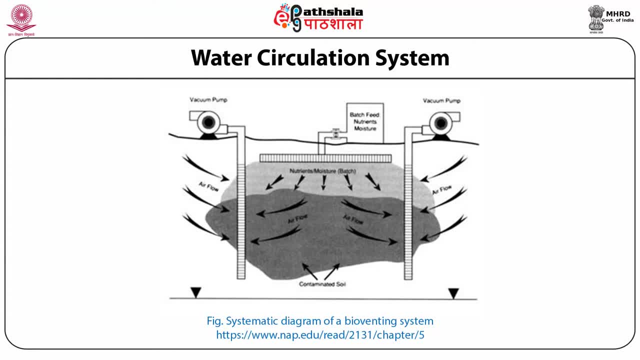 with the help of vacuum pump. then microbes are used in the developed or the aerobic bacteria developed at the site and they are removing the feed, nutrients and moisture. they are absorbing and removing the gaseous as a byproduct and the whole soil is cleaned by using the method of bioventing. 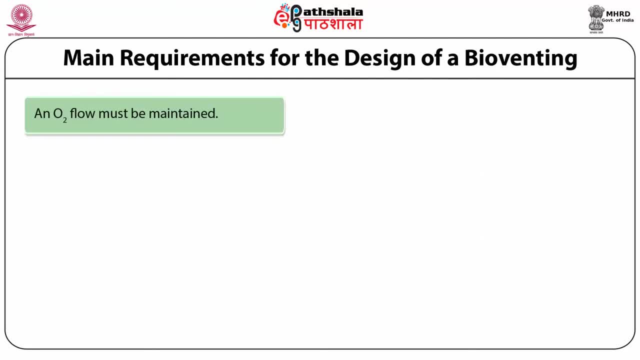 The main requirements for the design of a bioventing, including an oxygen flow, must be maintained through the contaminated zone at a level sufficient for the aerobic biodegradation of contaminants. Then the moisture of the soil should be maintained at an optimum value for microbial activity. 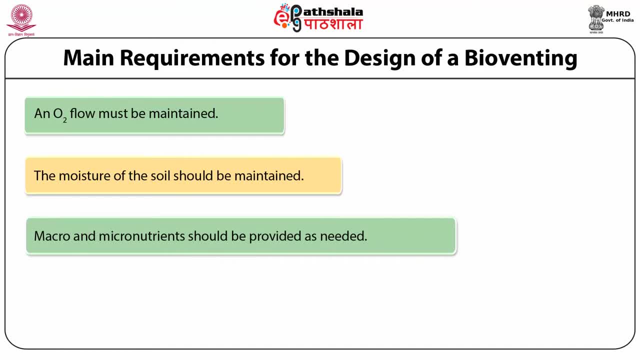 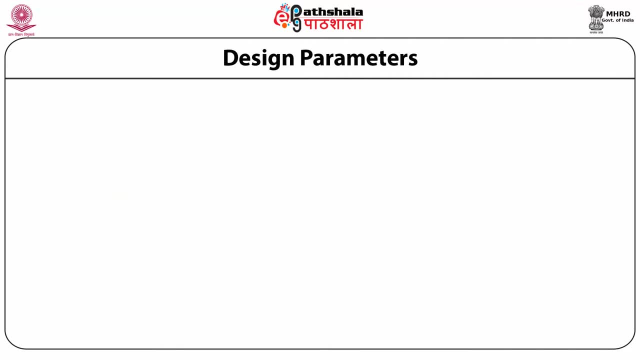 Then macro and micronutrients should be provided as needed. Now we discuss here about the designing parameters of bioventing. The most important design parameters are the including zone of influence, then the depth of air injection and the air injection pressure and flow rate. 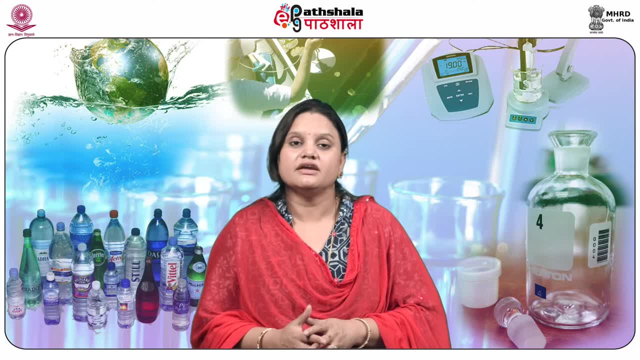 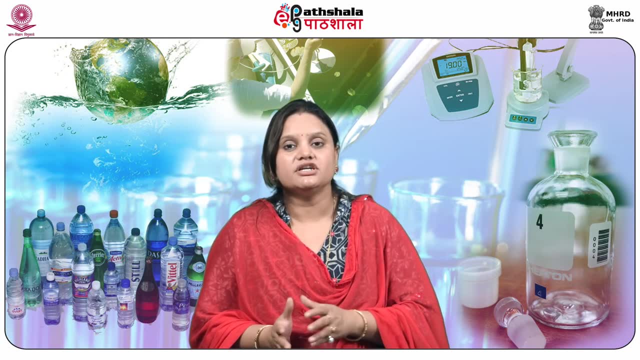 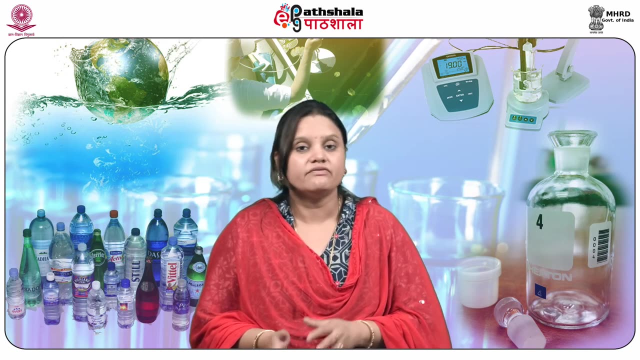 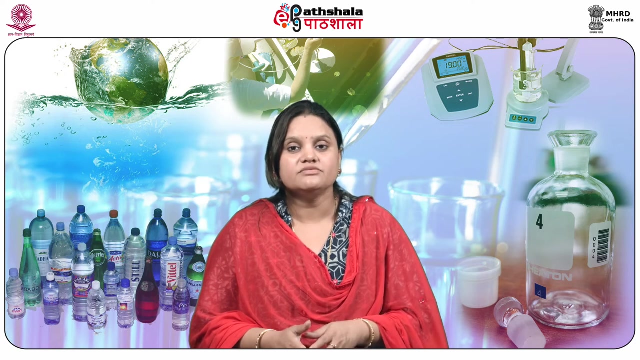 The next procedure we are discussing here is the bioaugmentation. The bioaugmentation constitutes of the addition of specific microorganisms to the polluted site. that includes soil or the water. When the pollutants are very complex and native soil microorganisms are not capable of degrading them, then additional microorganisms- 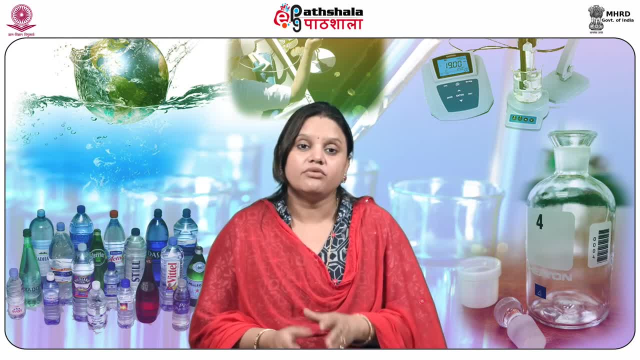 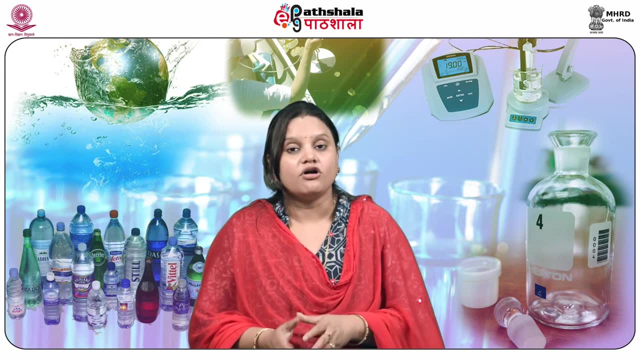 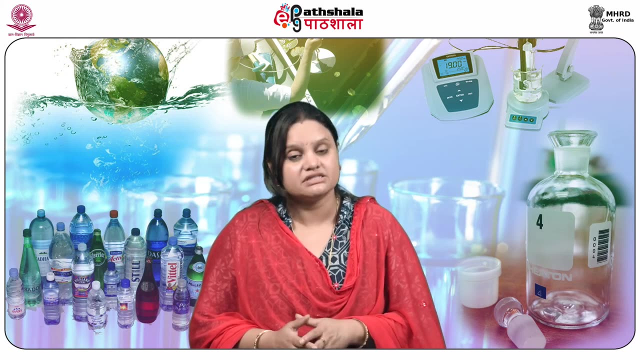 are introduced to the biodegraded pollutants, For example polychloro biphenyls, then trinitrins, then microtolvin, that is, TNT and the polyaromatic hydrocarbon. pesticides are degraded by using this technique: The seeding of microorganisms. 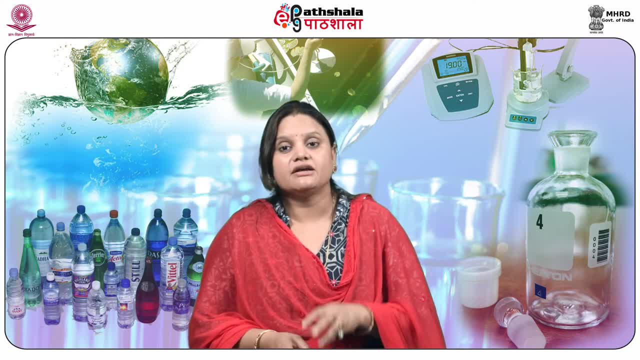 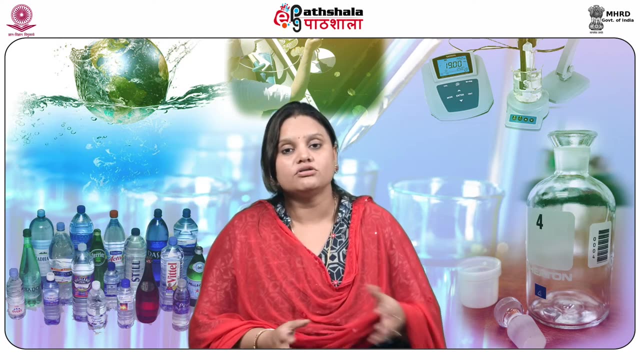 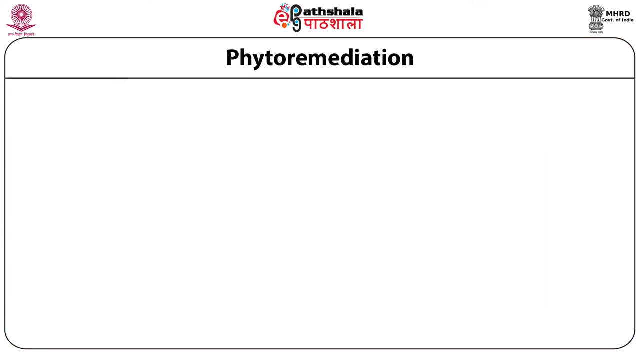 augments metabolic capability of indigenous microbial population. The introduction of microorganisms increases the rate or extent of degradation, or both, of the pollutants that may not be degraded by indigenous microflora. The next procedure that we are going to discuss here is the phytoremediation. 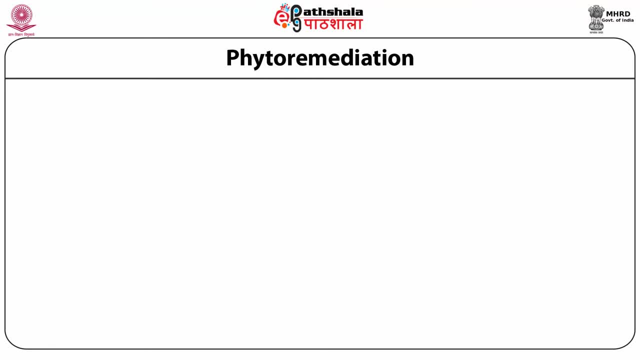 The phytoremediation is the use of green plants and their associated microorganisms and agronomic patterns to remove the pollutants or to make the environment free of pollutants. Plant roots absorb the pollutants and remediate them by accumulating the pollutants in the plant tissue. 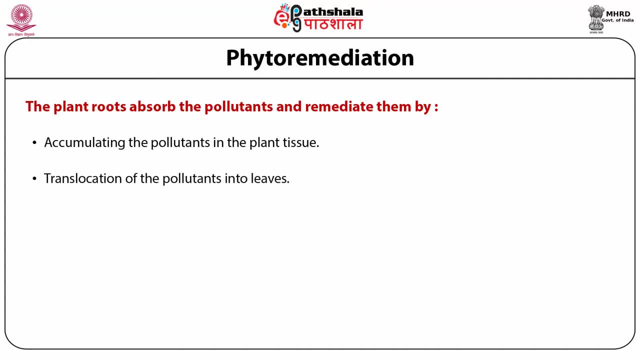 translocation of the pollutants into leaves and volatilization from leaf surface, then metabolism in rhizosphere, then degradation by microbial communities associated with plants and degradation by enzymes secreted by plants. Phytoremediation has been achieved for certain pesticides like 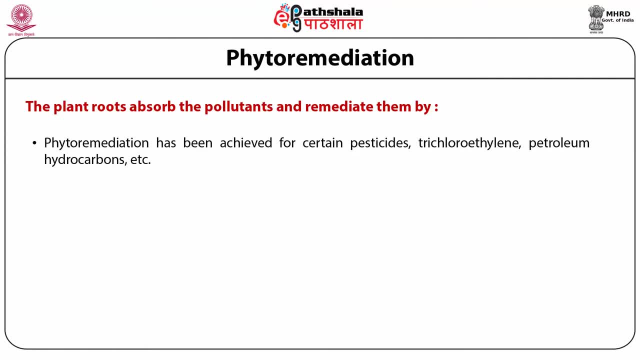 trichloroethylene, petroleum hydrocarbons, etc. However, the overall degradation or the remediation is relatively slow. If plants accumulate the pollutants, the plant's biomass has to be removed and appropriately disposed of. For example, carrots are used to absorb DDT. 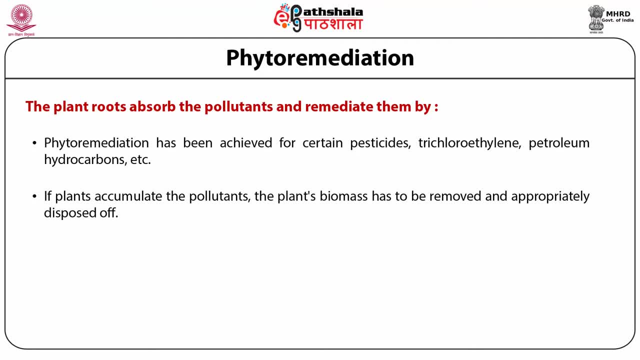 and these carrots are harvested, air dried and incinerated to decompose DDT. The transgenic plants may also be used. For example, Arabidopsis thaliana, which absorbs mercury, has been introduced and incorporated with genes coding reductase. 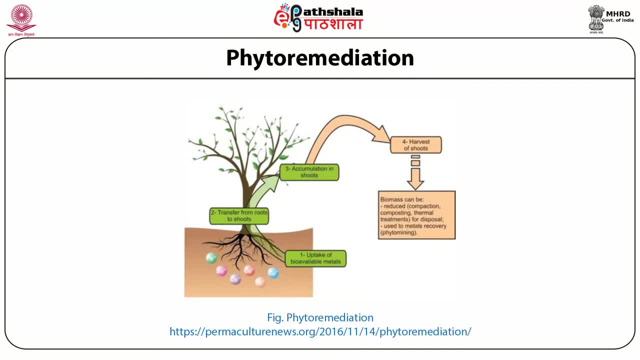 Here in this picture we are showing the process of phytoremediation, As we have seen in the picture that when the plant grows, it uptakes the bioavailable material from the soil, then transfers it from the root to shoot. 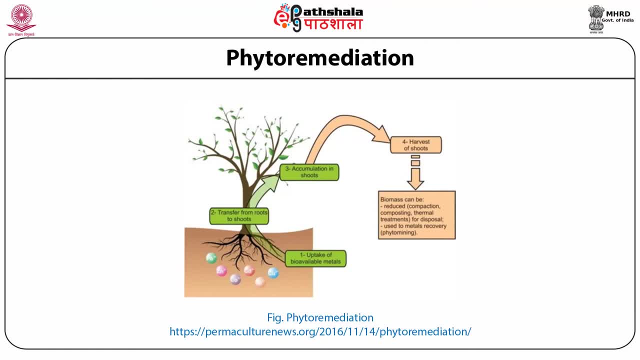 and then accumulation is done in the shoot part or the leaf part. then harvest these plants and then biomass can be reduced by compacting, composting or the thermal treatment, or it is disposed of by using the metals recovery or the phytomining. 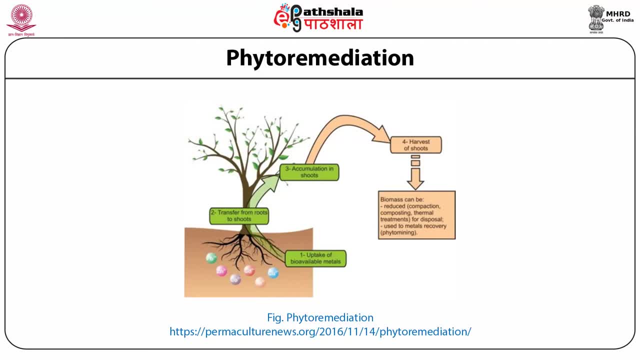 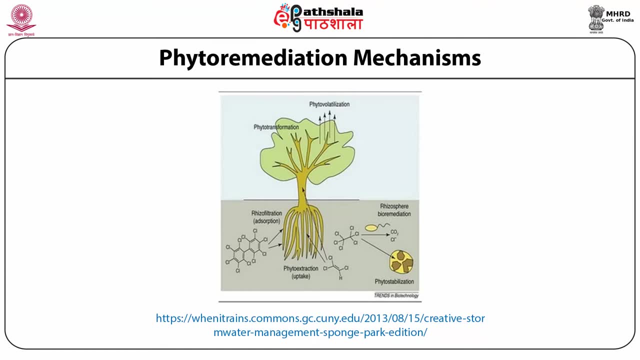 In the next picture we are again. this picture shows the phytoremediation mechanism. Here the various methods are going out in the different plants of the parts of the plant. This shows that at the root level the phytostabilization 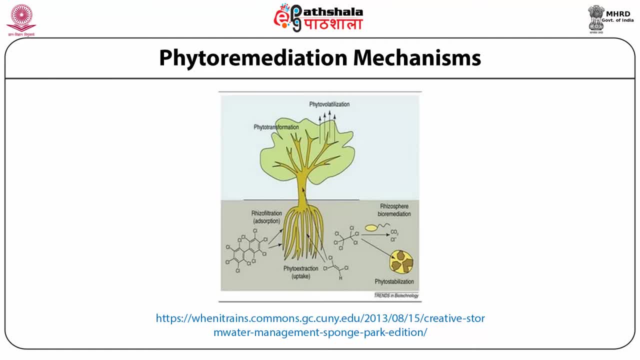 and phytostimulation process is continued, that the pollutant is immobilized in the soil. Then, after the pollutant becomes immobilized, then the phytoextraction, like the pollutants accumulate in the harvestable parts of the tissue, is done by this process. 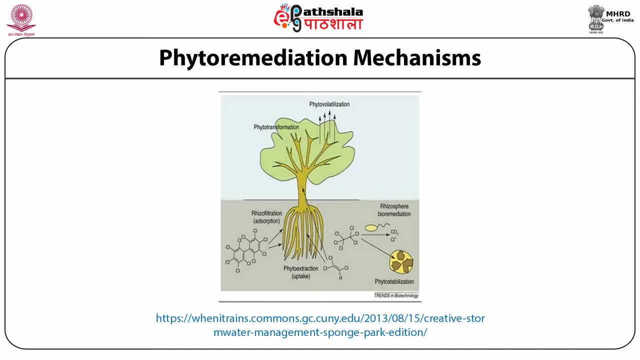 Phytovolatilization is also done in the same part. by this process the pollutants is released into the atmosphere, into the volatile form. Simultaneously, the phytodegradation- it means the utilization of the pollutants at the leaf level- is also carried out. 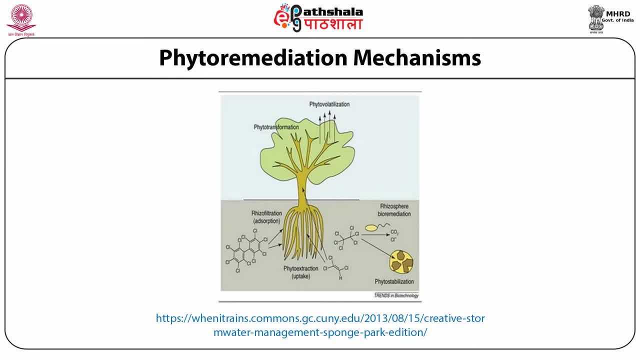 due to the phytoremediation procedure, The main processes, including the phytoextraction, then rhizodegradation. the rhizodegradation is carried out at the root level of the plant, where the rhizomes are degrading the existing pollutant. 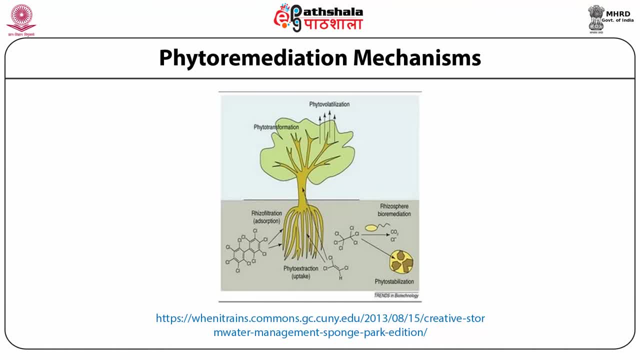 in the soil. Then the phytodegradation again is the same process, that is carried out at the root level, then phytovolatilization is done by the either shoot level or the leaves level, then the phytostabilization that is also done in the 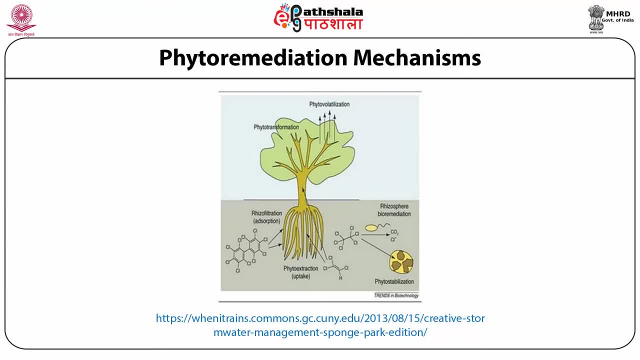 roots of the plants, and the rhizofiltration is also done in the root part, where the rhizomes of the roots filtrate the pollutants from the soil. Here, in this figure, we are discussing the air sparging method. in this method there are the vacuum pump. 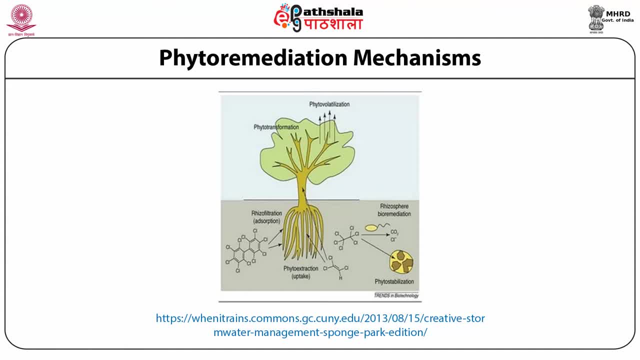 and the compressor which provides the force air flow deep into the contaminated soil. then the air flow mixed with the contaminated soil and the microorganisms are developed with the help of nutrients and the moisture so that they are synthesized their food with the help of the pollutants present in the soil. 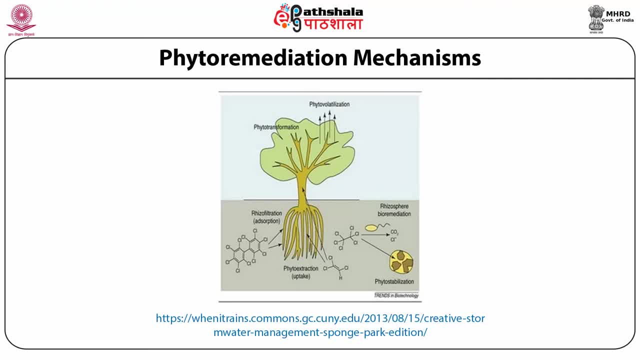 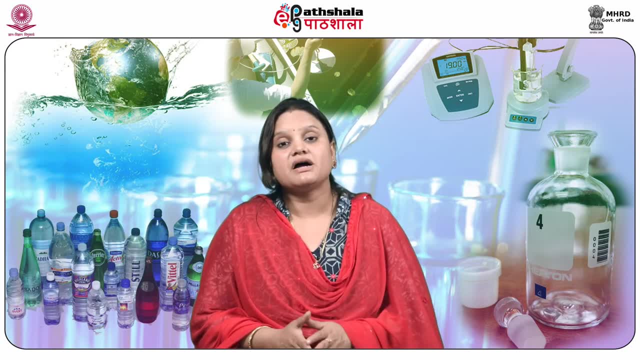 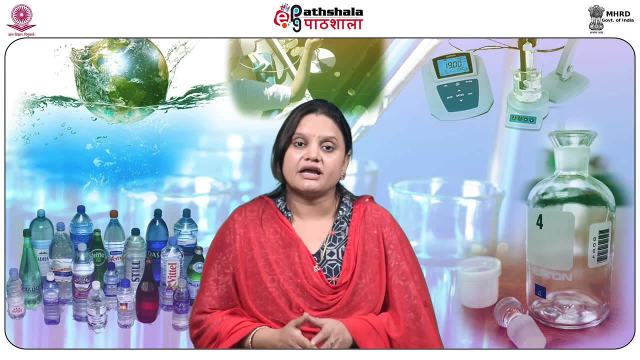 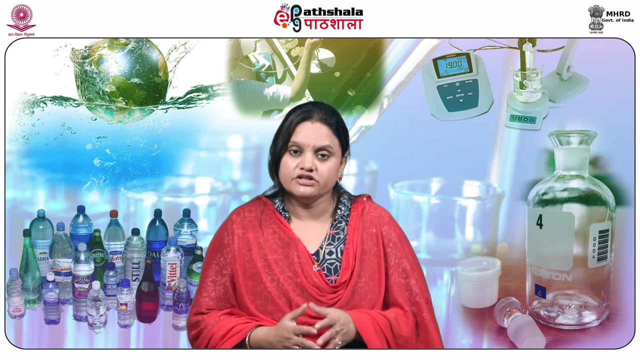 and the soil is decontaminated by this process. now we are discussing here the method bio-sparging. bio-sparging is an in-situ bioremediation technique that uses the indigenous microorganisms to degrade the pollutants in saturated zone in bio-sparging oxygen. and the nutrients are injected into a saturated zone to increase the biological activity of indigenous microorganisms. the bio-sparging can be used to reduce the petroleum products that are dissolved in ground water or adsorbed to the soil below water level. it is more effective to remove pollutants. 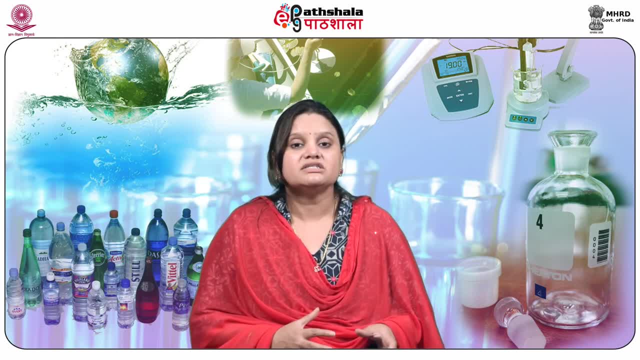 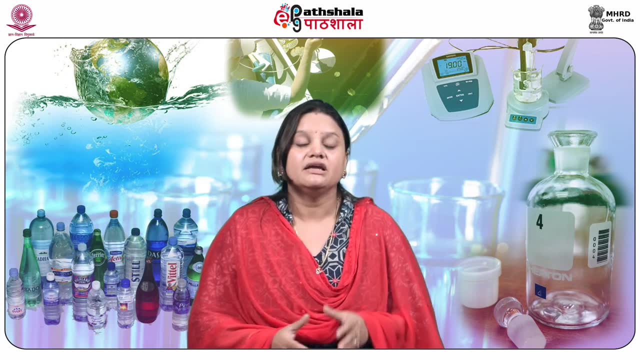 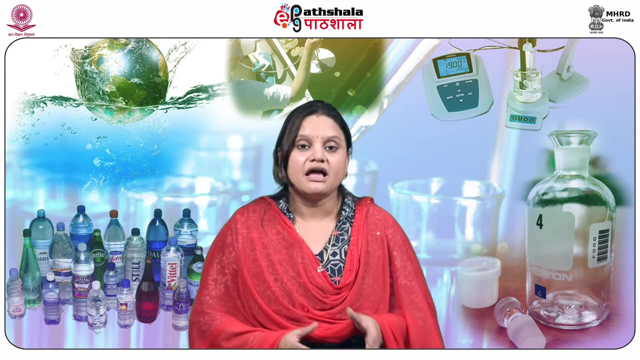 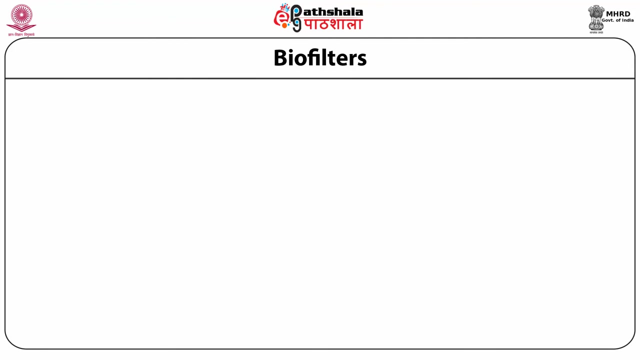 in saturated zone. the bio-sparging is most effective at site with the medium weight petroleum products like diesel, kerosene, etc. bio-sparging promotes the biodegradation and the process is similar to the bio-venting. now the next procedure is known as bio-filters. 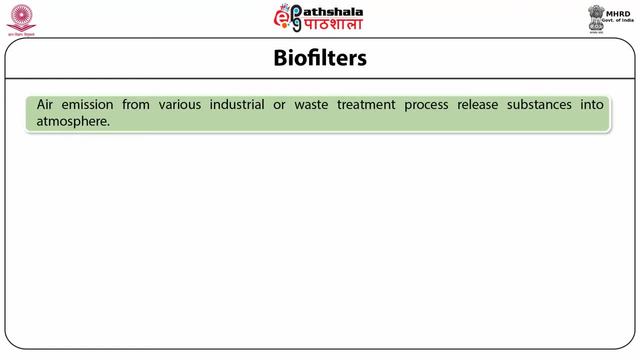 the air emission from various industrial or the waste treatment process release substances into the atmosphere that may be hazardous to human. the air emission can be controlled by various physicochemical means, such as condensation, scrubbing, adsorption, etc. however, these processes are costly and difficult to operate. 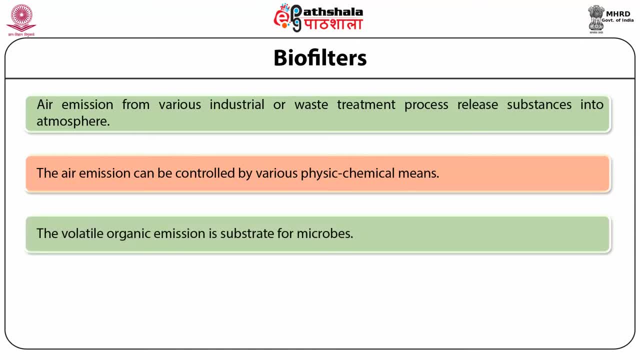 the volatile organic emission is substrate of for microbes, hence the use of micro organisms through bio-filters like trickling bio-filters and bio-scrubbers. the bio-filters are the solid surfaces with microbes grown on them that are able to degrade the pollutants. 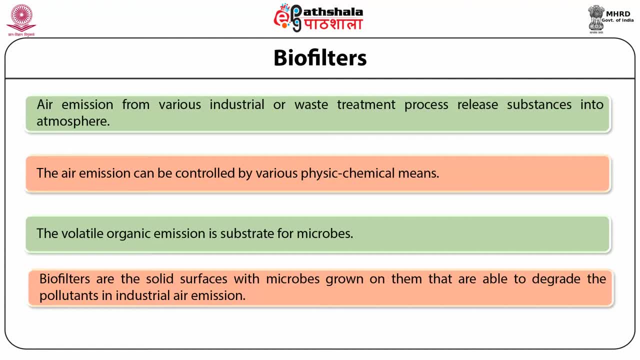 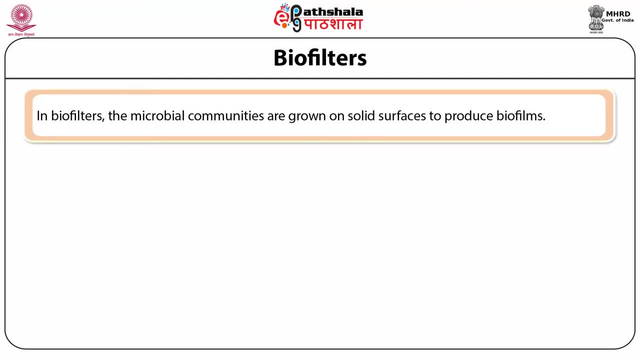 in industrial air emission. in bio-filters, the microbial communities are grown on solid surfaces to produce bio-film. when the gas stream containing organic pollutants are passed through these systems, the pollutants are adsorbed onto the bio-film. the micro-organism are immobilized on a. 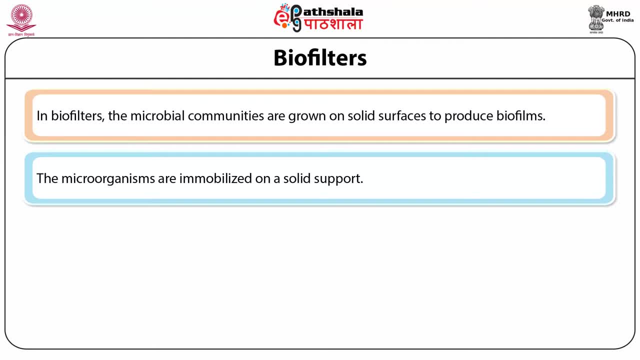 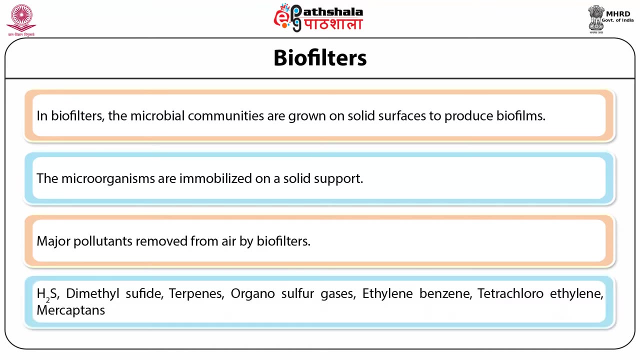 solid support and the classical bio-filter use composed soil, bark, peat, etc. as a filter media. the major pollutants removed from air by the use of bio-filter: the hydrogen sulfide, dimethyl sulfide, terpenes, organic sulfur gases, ethylene, benzene, tetrachloroethylene. 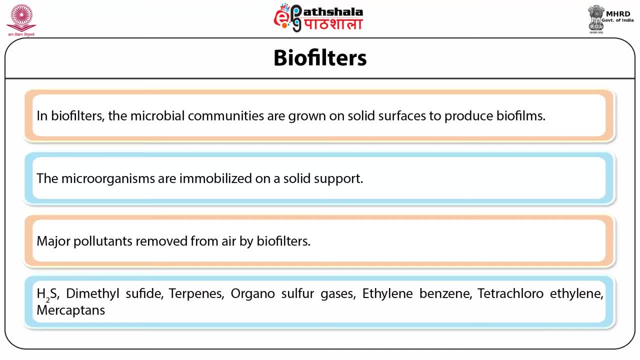 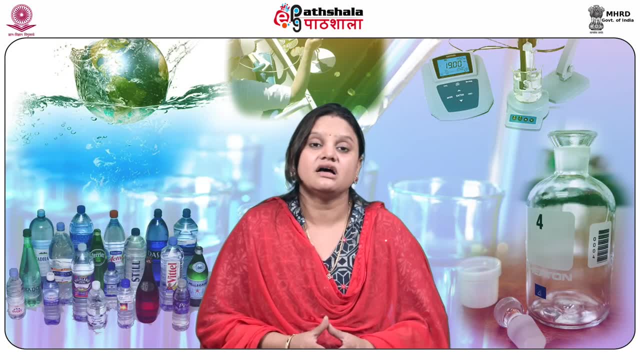 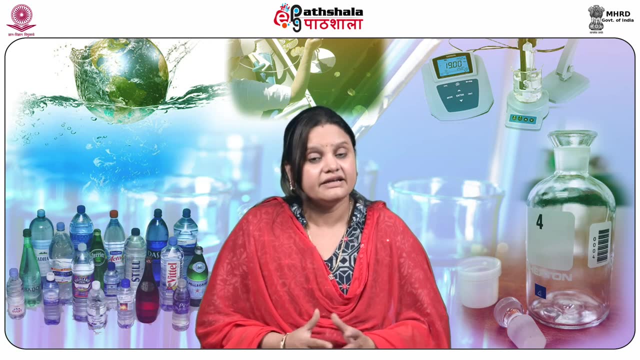 and mercaptan are some example of pollutants that removed by the bio-filters. now the next technique that we are going to discuss here is the ex-situ bioremediation or off-site bioremediation techniques. it is the bioremediation. 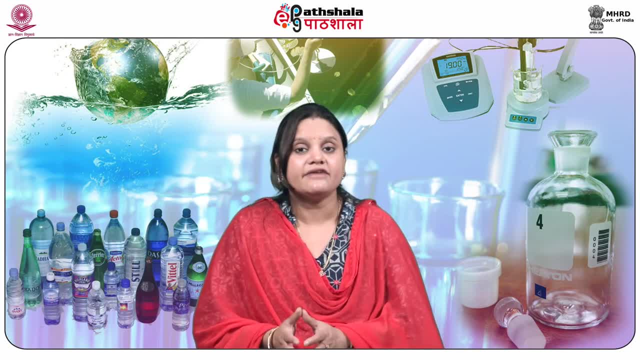 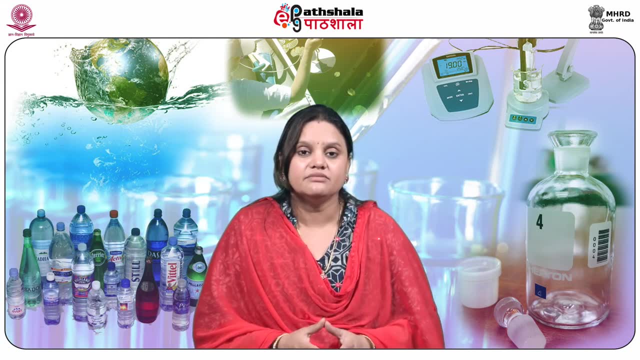 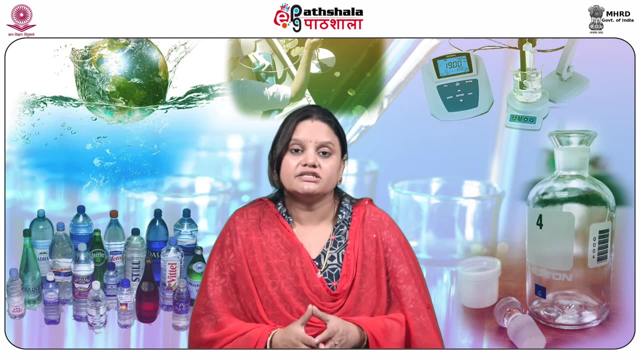 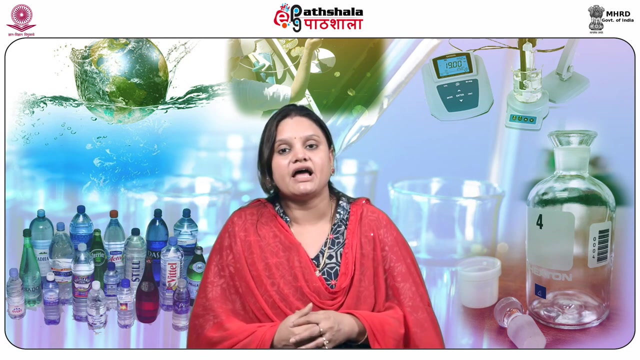 in which the polluted material are collected from the polluted site and the bioremediated with the requisite micro-organism- that is known as the consortium of micro-organism- at the designed place or the site. this has been successfully applied for the bioremediation of soil. 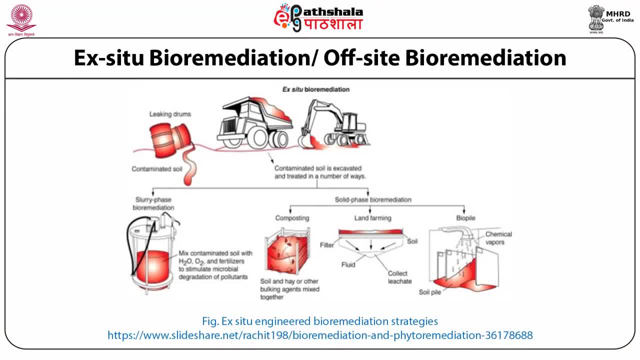 and water. this picture shows the ex-situ engineered bioremediation strategies. here we have seen that the soil is contaminated by leaking some drums of chemicals or the petroleum products. then the contaminated soil is excavated and treated in a number of ways, which includes the slurry phase bioremediation. 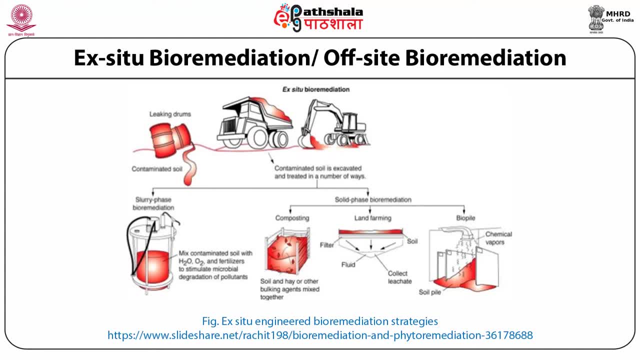 or the solid phase bioremediation. in the slurry phase bioremediation, the soil or the contaminated soil mixed with the water, oxygen and the fertilizer to stimulate microbial degradation of the pollutants. and in the solid phase bioremediation, three processes are carried out. 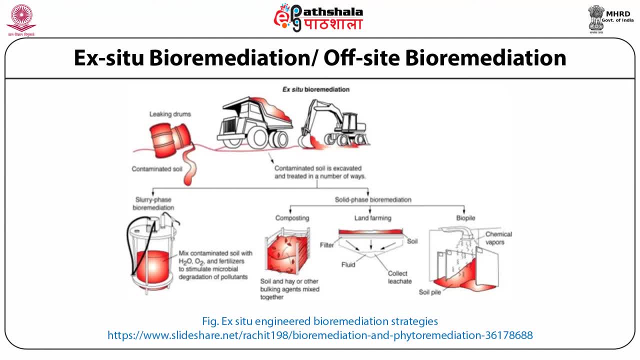 including the compost composting land farming and the biopile. in the composting, the soil and the hay of the other bulking agent mixed together to convert it into the manure or convert the natural fertilizer. then the land farming, including the soil, is transferred into a 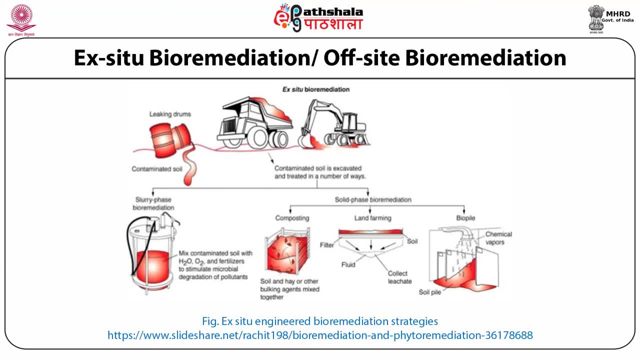 particular land where the filter and flutes are present to collect the leachate of such kind of pollutants. then the biopiles, including the chamber of the soil pile which is sprinkled by the chemical vapors so that the chemicals or the pollutants present in the soil is. 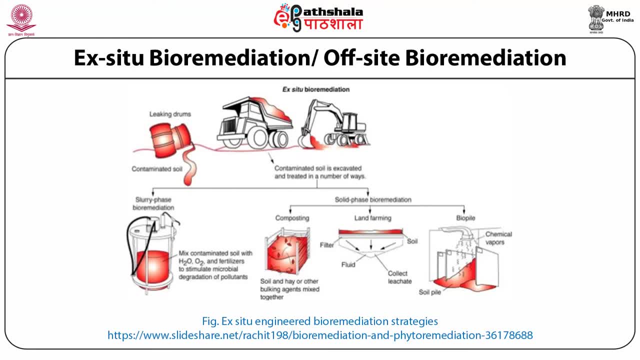 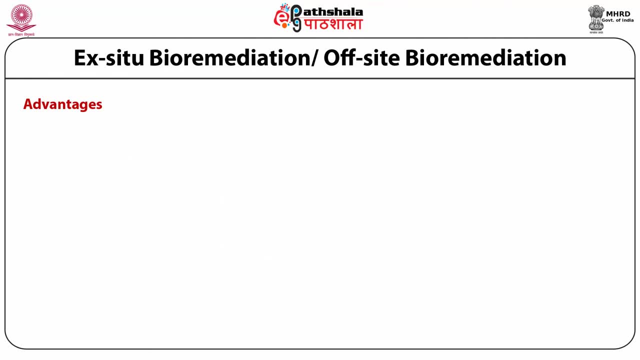 react with such chemical vapor and removed from the soil. the advantages of using this method is that it is better controlled and more efficient method. it takes short time to remediate the soil, comparative to the in situ method, and the process can be improved by enrichment with the. 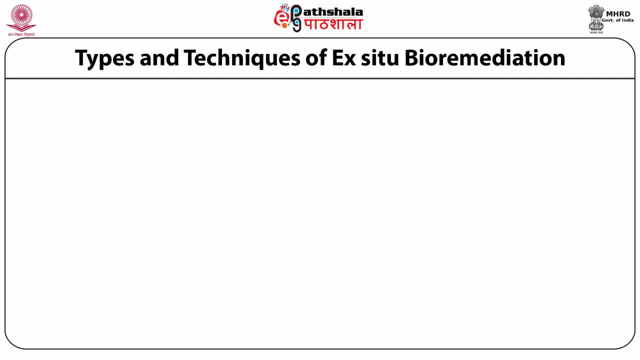 microorganism. now we discuss here about the types and techniques used for ex situ bioremediation. the first method is land farming. it is also known as BTX. the land farming is an above ground remediation technology for hydrocarbon like petroleum, contaminated soil through the 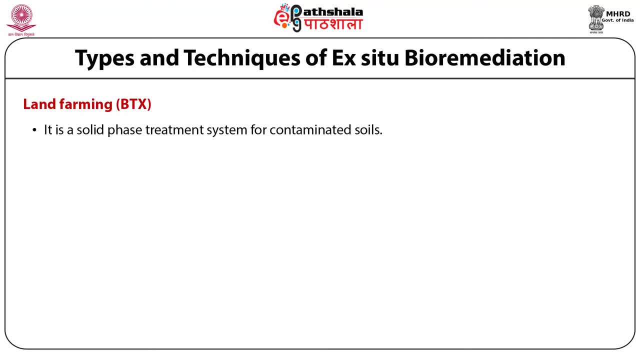 biodegradation. it is a solid phase treatment system for the contaminated soils. in this technique, the contaminated soil is excavated, mixed with microorganisms and nutrients and spread out on the ground surface or the liner. the soil is regularly turned for mixing and aeration. the efficiency of 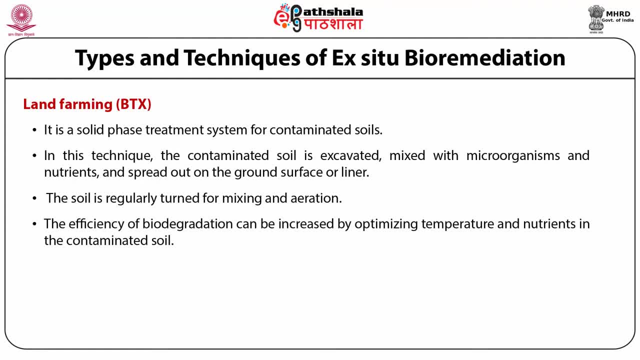 biodegradation can be increased by optimizing temperature and nutrients in the contaminated soil. the addition of coarse substrates and anaerobic pretreatment of the soil also enhances degradation processes. the land farming has been successfully used for the bioremediation of benzene, toluene and 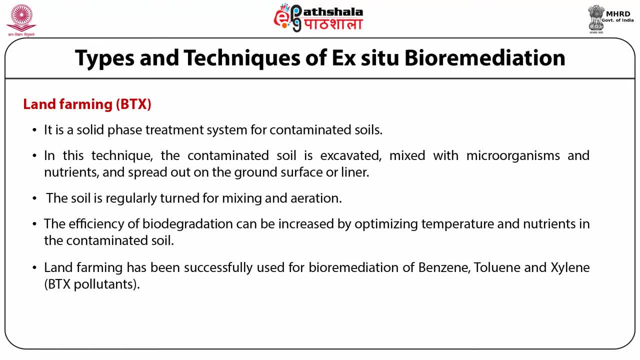 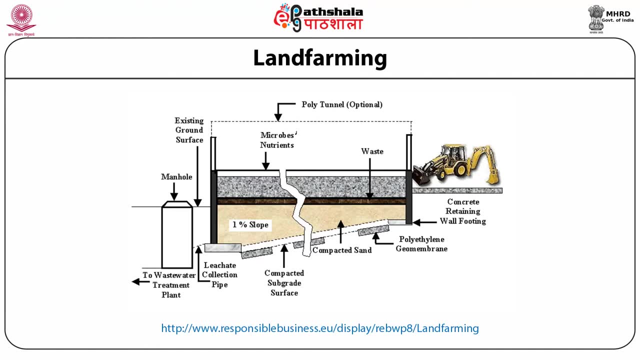 xylene. that's why its name is denoted as BTX. that is the initial of benzene, toluene and xylene, which are very well known as BTX pollutants. here is the picture of land farming. in this picture, the polytunnel or the 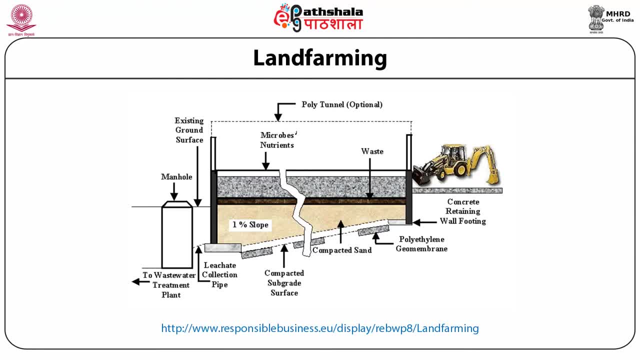 microbes, nutrient and the waste is transferred to the portion where the soil is bioremediated. then the concrete retained wall footing is developed because this soil is not contaminated the other soil of the same land. then this ground level is developed, compacted by the sand or the polyethylene. 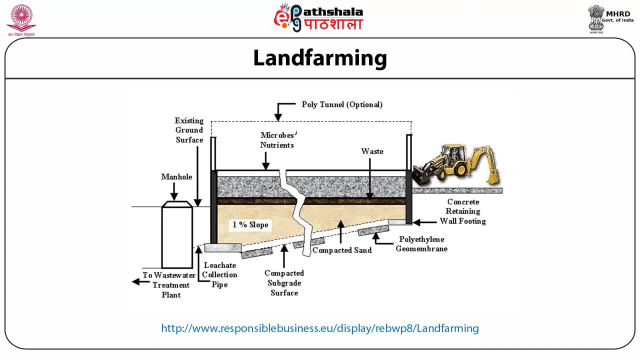 geomembrane. so when we applied the waste water, either the existing ground surface is transferred to the main hole, which is again transferred to the waste water treatment, but when we doing the land farming here, then the microbe nutrients or the waste is mixed with the soil particle. 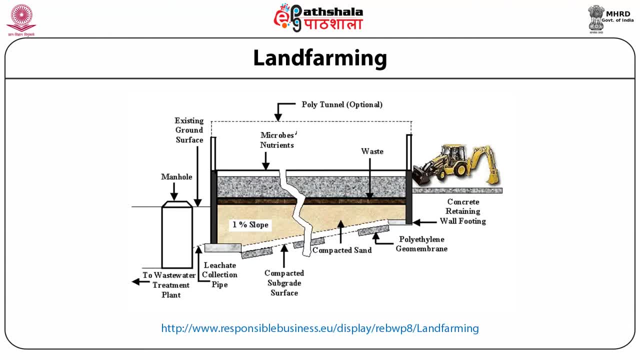 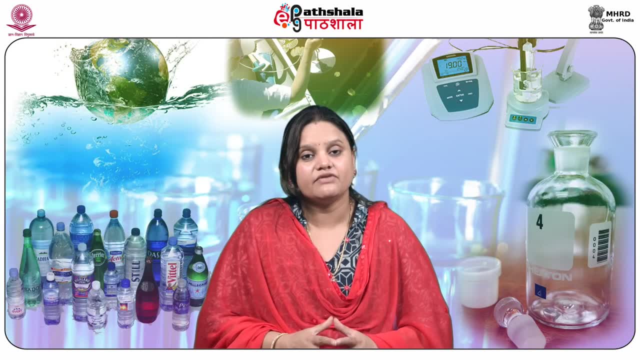 so that they are degraded, the pollutants, particularly benzene, toluene, xylene, from the soil. now we are discussing here another one ex-situ technique, that is, composting, or we are also known this technique as a biopiles. the composting is the anaerobic. 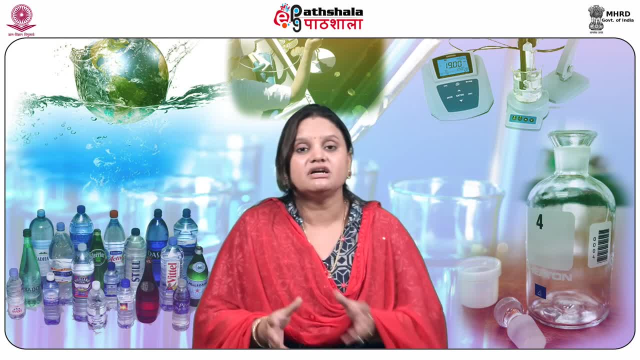 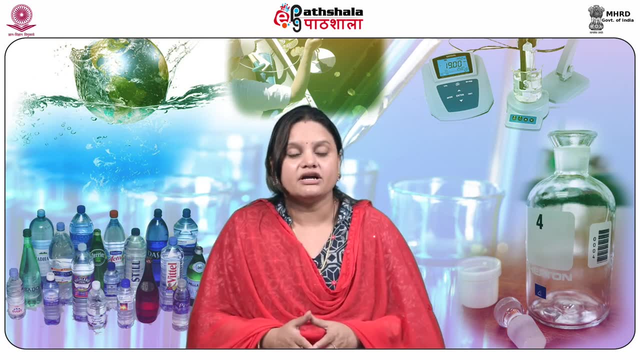 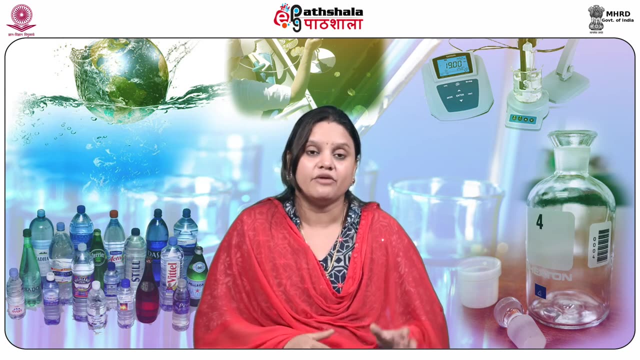 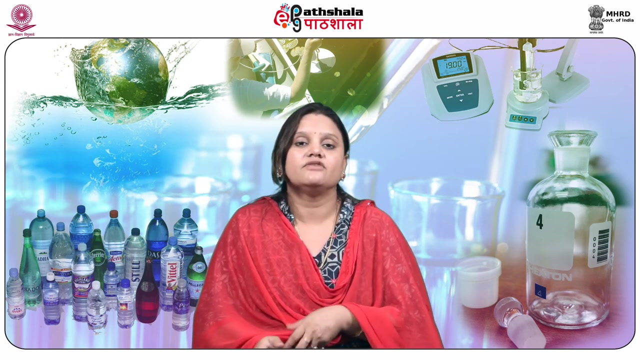 thermophilic process of microbiological degradation of contaminated material like organic waste, to stable ant products that are usually compost and that can be safely disposed of into the environment. it is controlled biological process by which organic contaminants are converted by the microorganisms to safe established by products. 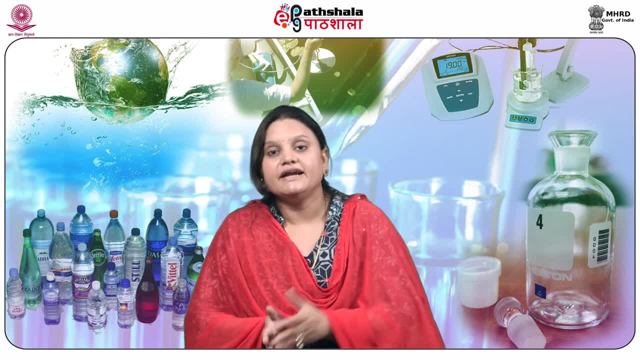 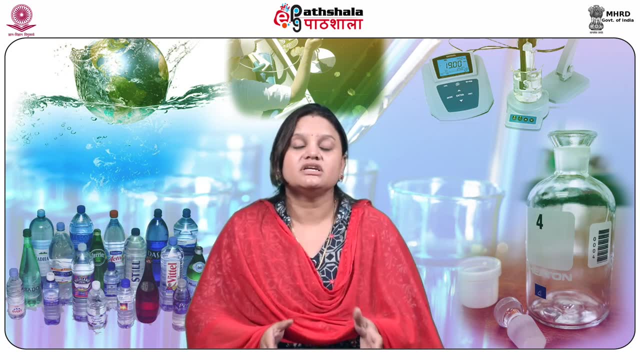 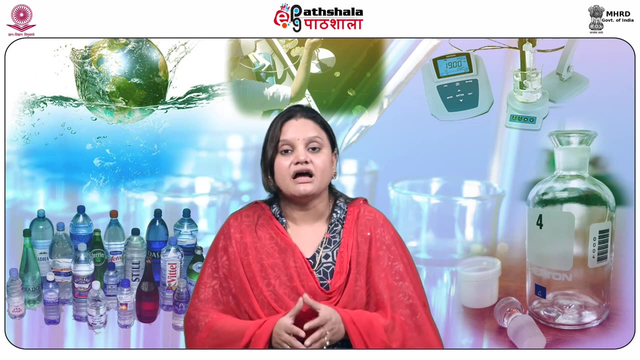 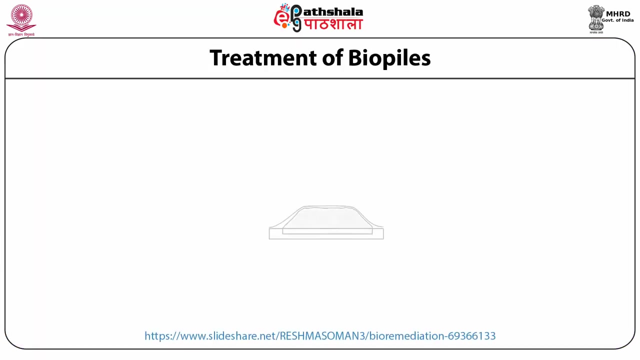 the contaminants are degraded, typically under a thermophilic conditions. in most of the cases, the composting is achieved by the use of indigenous microorganisms, the waste that are established to less complex material with the decrease in their masses. this figure shows the treatment procedure through the biopiles. 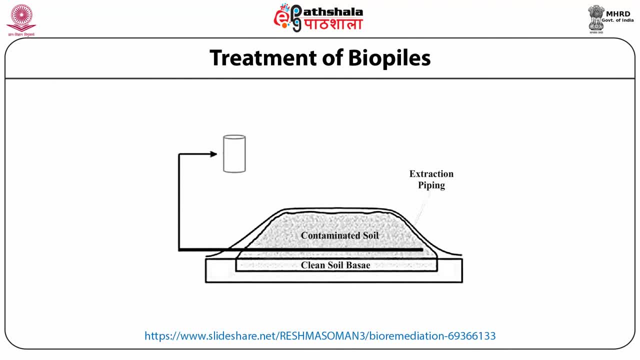 or the compost method. you have seen that the clean soil base, the contaminated soil prepared bag of contaminated soil, then the condensation and collection tank is prepared where, when the contaminated soil is treated with the microorganism that they are converting the anaerobic bacteria developed here and by the 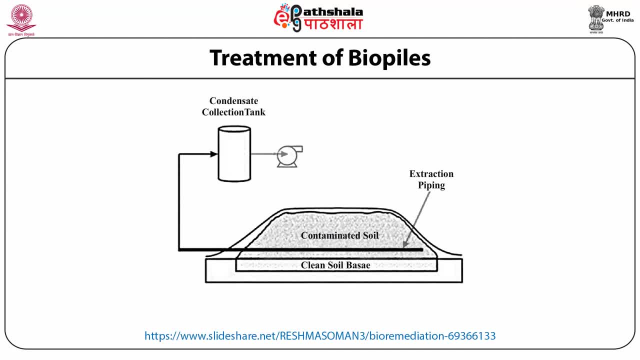 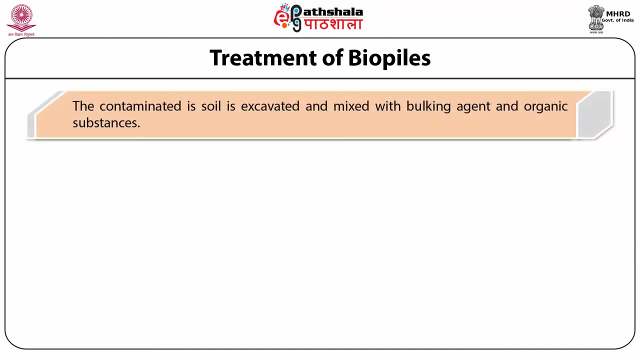 thermo process. these bacteria convert the pollutant into the stable and products that are generally the compost, which is again transferred to the condensation and the collection tank, and the gas which is released from this process is, after the treatment, release into the atmosphere. the contaminated soil is excavated. 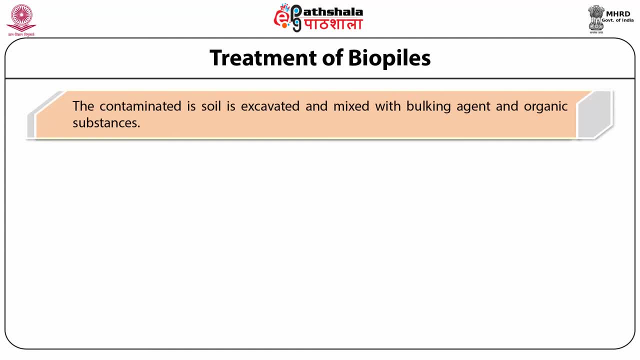 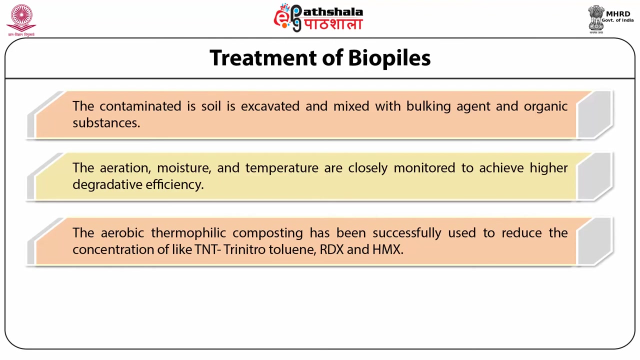 and mixed with the bulking agent and organic substances like wood chips, animal waste, vegetative waste, etc. the aeration, moisture and temperature are closely monitored to achieve higher degradative efficiency. the aerobic thermophilic composting has been successfully used to reduce the concentration of TNT. 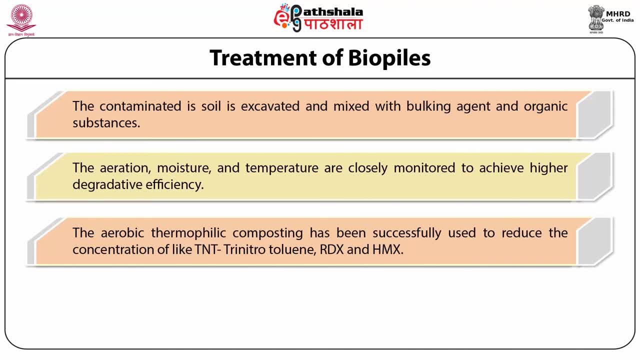 like this is 3-nitrotolvane, RDX and HMX, then the composting has also been used to treat sewage sludge, soil contaminated with diesel, waste from bruise, antibiotics, fermentation waste and waste from the processing units. methods of composting included windrows. 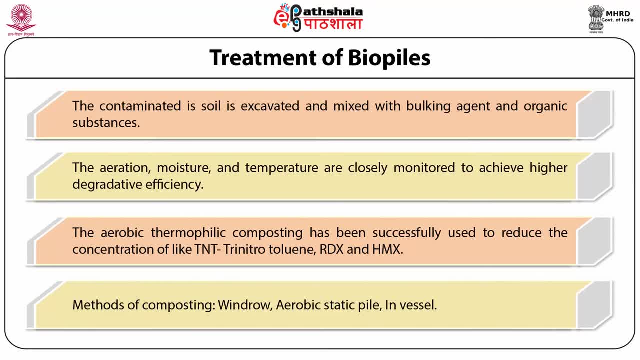 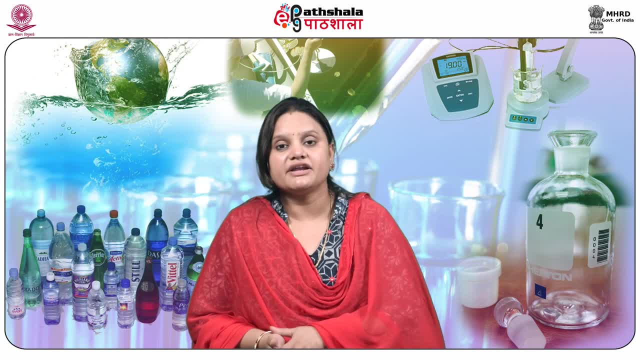 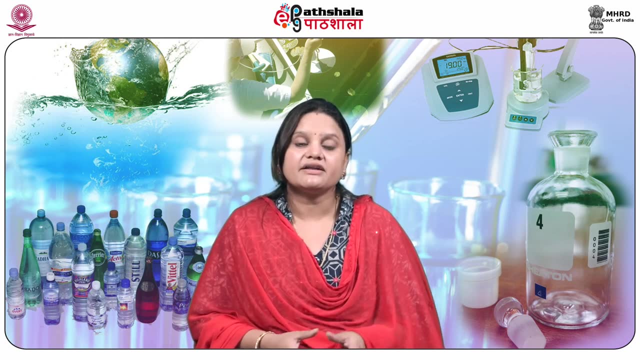 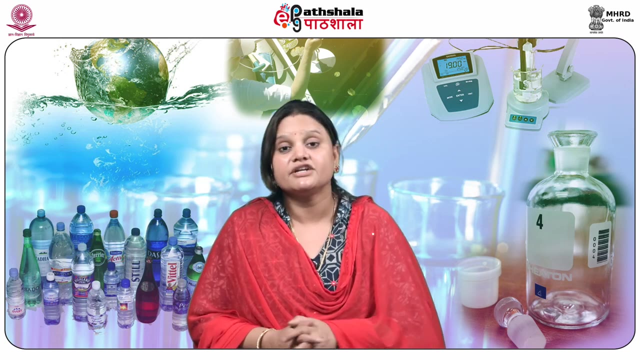 aerobic static pile and in vessels. now the next method is bioreactors. in this approach, the biodegradation of the contaminants is carried out in a large bioreactors. the bioreactors can be used to treat liquid effluents or contaminated solid waste. the contaminated solids 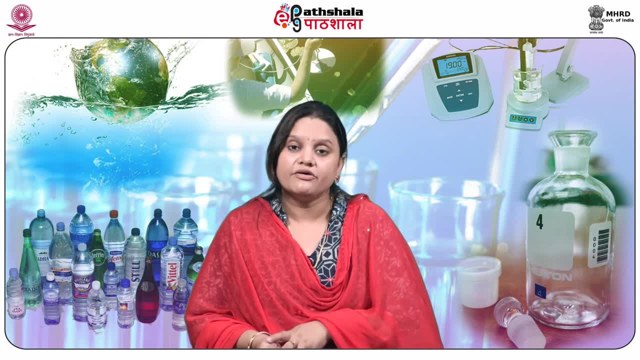 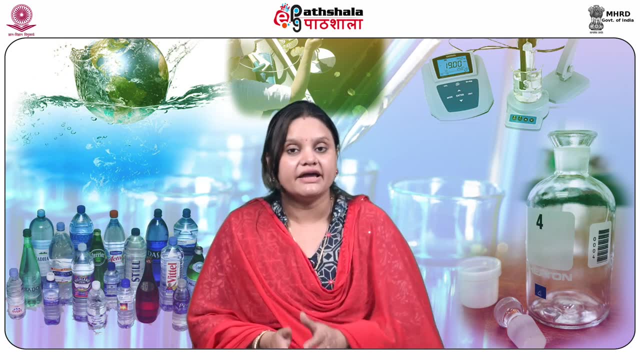 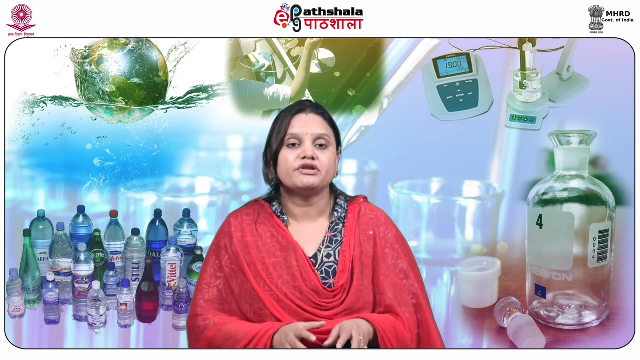 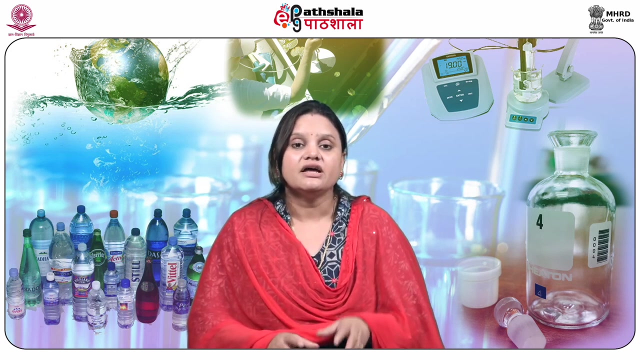 or the liquids are subjected to bioremediation under the controlled condition in specifically designed bio aerator. the nutrients, supply, temperature, aeration, moisture, contact between the microorganism and the pollutants, etc. are maintained at optimum condition. hence the degradation is very rapid and efficient. however, running 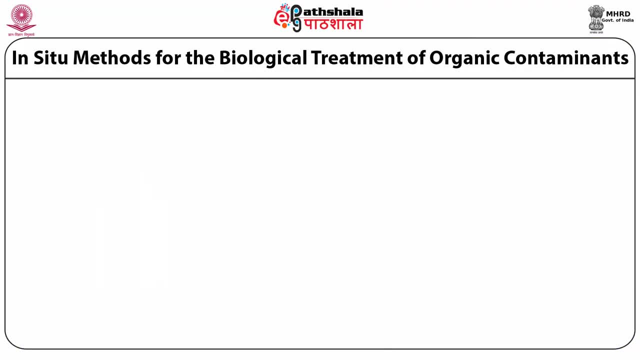 cost of bioreactor is very high. the in-situ methods for the biological treatment of organic contaminants. first one is the bioremediation in the widow's zone. when the contamination exists substantially above the water table, that is in the widow's zone, a very efficient in-situ. 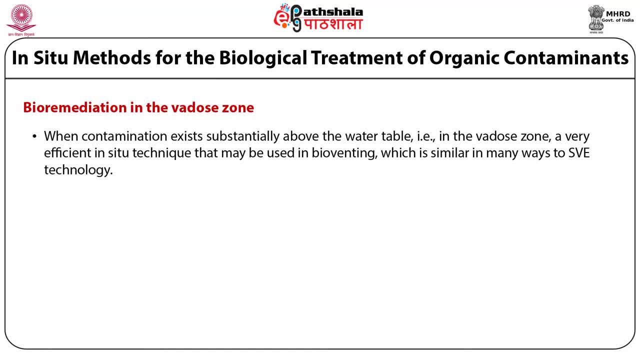 technique that may be used is bioventing, which is similar in many ways to SVE technology. the next one is the bioremediation in the water saturated zone. the two kinds of system are usually applied for it. the number one is water circulation system, where underground is pumped. 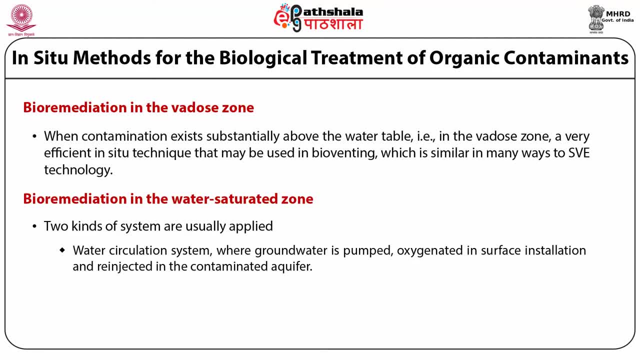 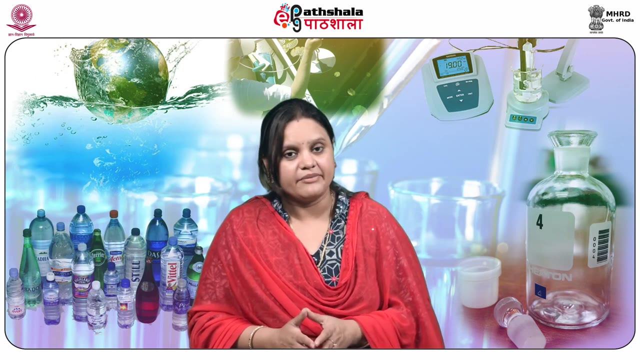 oxygenated in surface installations and re-injected in the contaminated aquifers. and the second one is the air sparging system, which involves the injection of air directly into the groundwater. here we are discussing about the examples of some microbes that are used in the bioremediation that 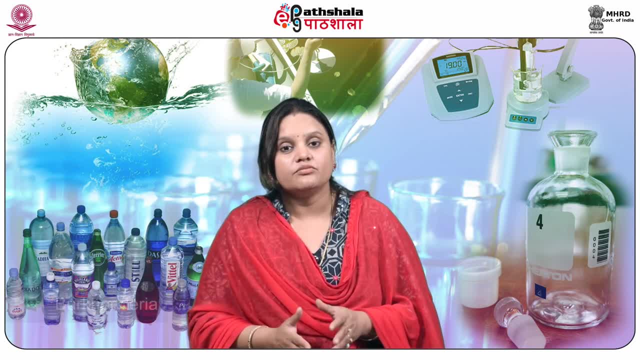 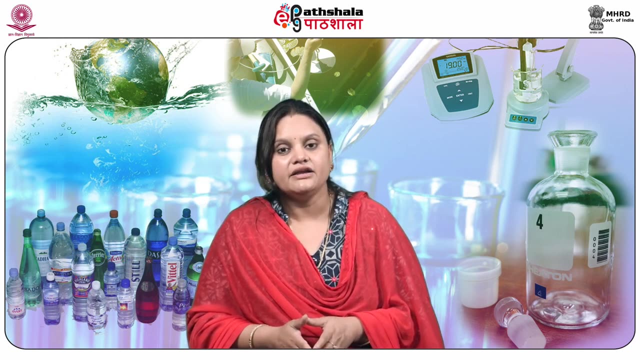 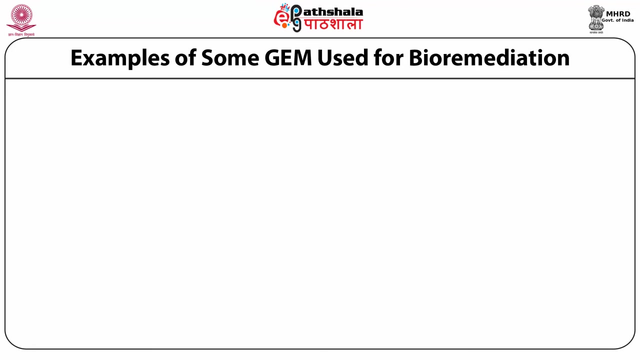 include Pseudomonas putida, then Bucureldaria, then Methyl Methylosinus, then Ralstonia, then Ecoli JM109, then Comemonas and Pseudo Pseudoallalkalogens. here we are discussing about some examples of some. 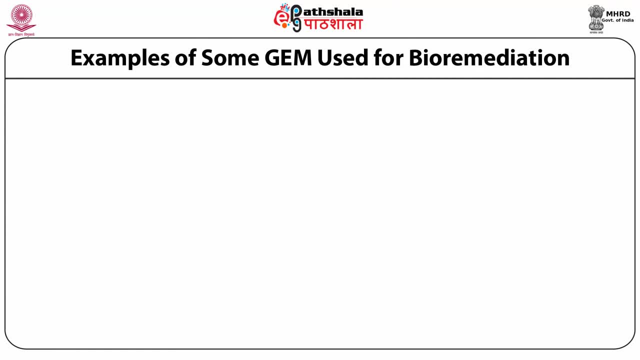 GEM, that is, genetically engineering modifier used for bioremediation. role of Dinococcus and Radiodurans in bioremediation is an important example of some GEM techniques. then the TOL, plasmid pathway of Pseudomonas putida. 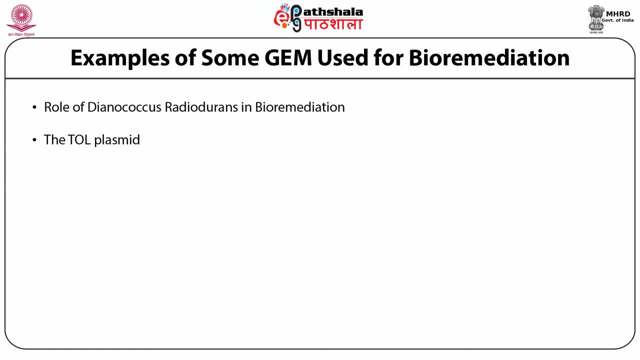 has been manipulated extensively to expand its catabolic capability on different branched compounds. the plasmid PWR1 or of Pseudomonas species B13 have been modified to generate hybrid pathways that extend vertical degradation of chlorinated compounds. Ecoli JM109. 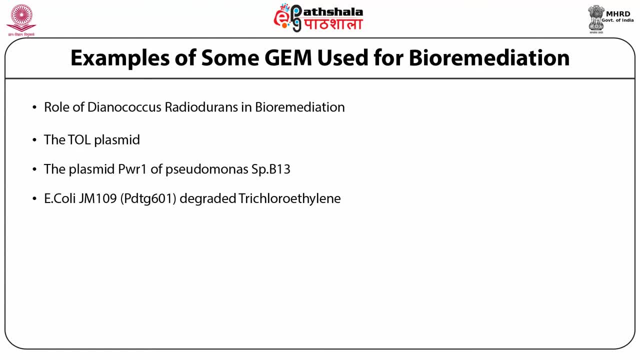 or PDTG 601, degraded trichloroethylene and aerobic bacterium Bucureldaria Cipacea. G4 degrades trichloroethylene to carbon dioxide and non-volatile products by toluene or monooxygenase. when TN5. 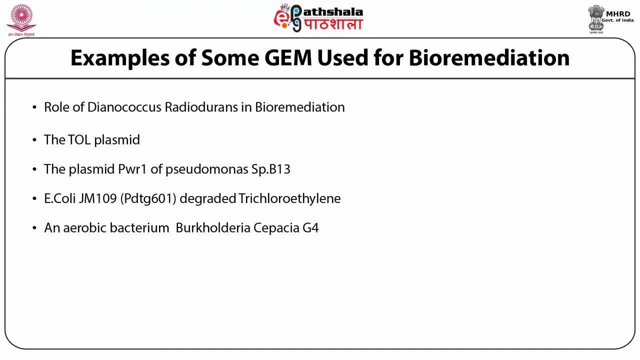 mutants of strains GA4 were constructed via triparental mating. the Ralstonia eutropha AEK301 produced via triparental mating and have lost phenol in the form of trichloroethylene in the form of trichloroethylene. 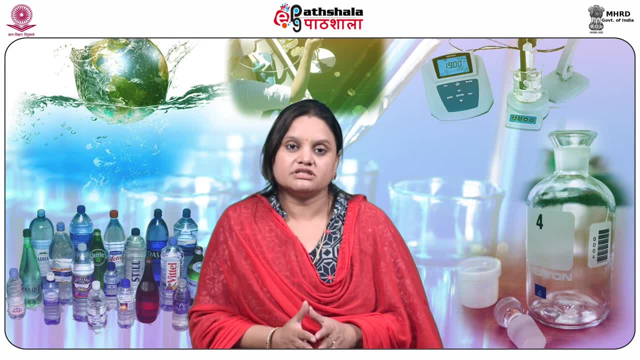 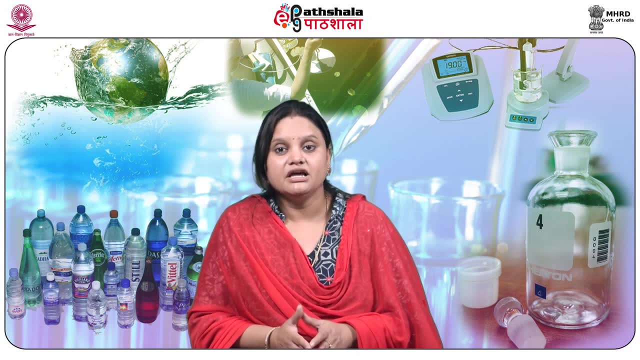 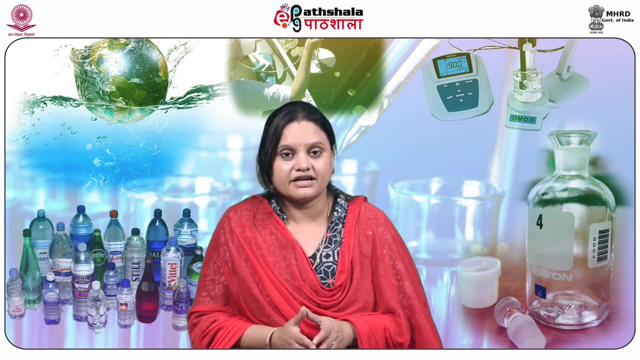 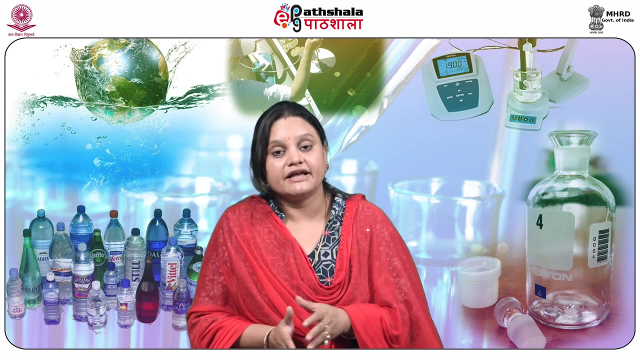 now we are discussing about the advantages of using the bioremediation process. there are a number of cost efficiency advantages of bioremediation. that includes, because it is a bioremediation method, the toxic chemicals are destroyed or removed readily by using the natural microorganism. 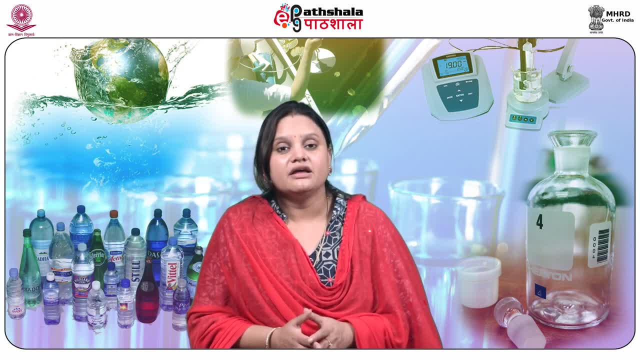 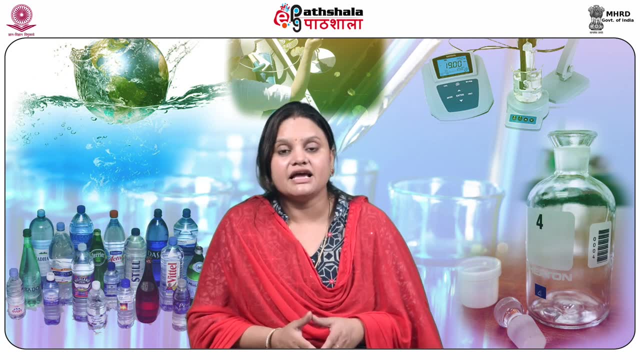 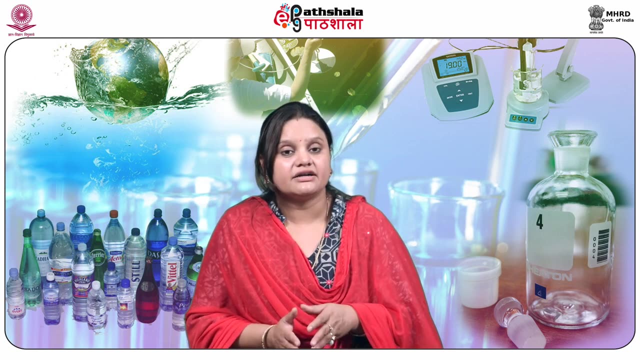 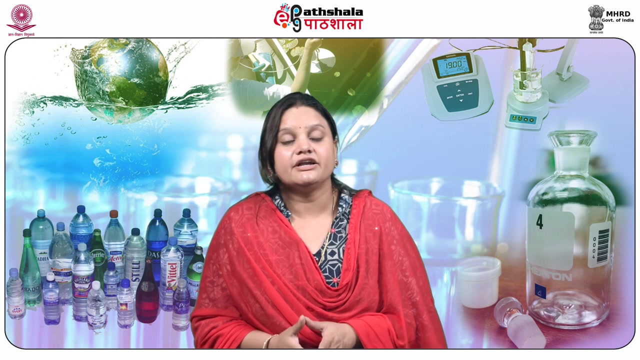 then these methods having a low capital expenditure and they required less manual supervision. these methods required less energy as compared to the other technologies and the genetically engineering modified in the bioremediation. now we are discussing here about some limitation and disadvantages of bioremediation.